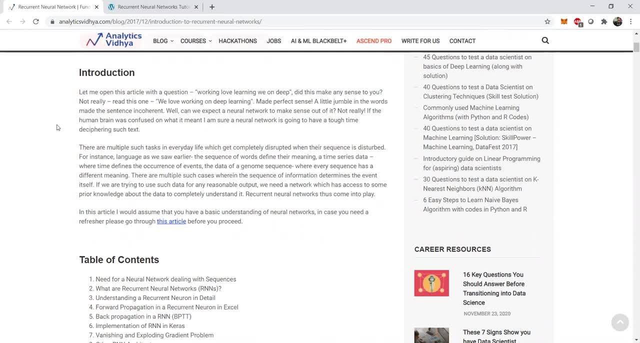 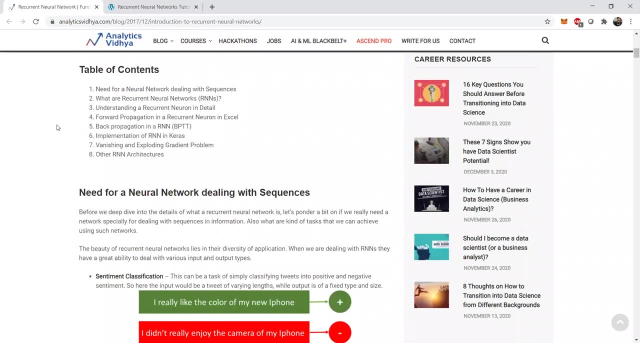 These set of neural networks are vastly used, mainly due to its memory retention, and also it can capture lots of information From a particular classification tasks or any tasks in general, particularly in the field of NLP. RNNs have made the breakthrough from a long time. 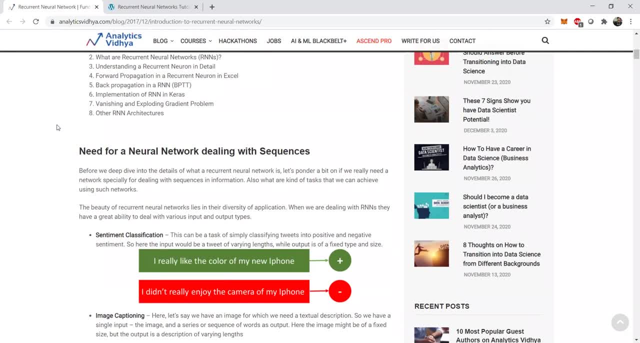 So, in the context of sentiment classification, The image captioning, everywhere we find that RNNs are always there. I'll beat in the present time. These are present in the form of sophisticated architecture, but the basic form of regular neural networks are still persistent, even to this day. 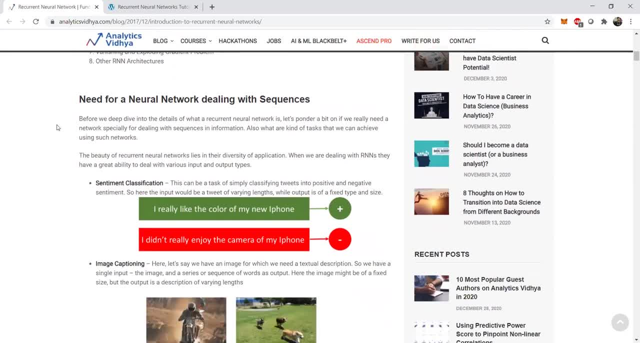 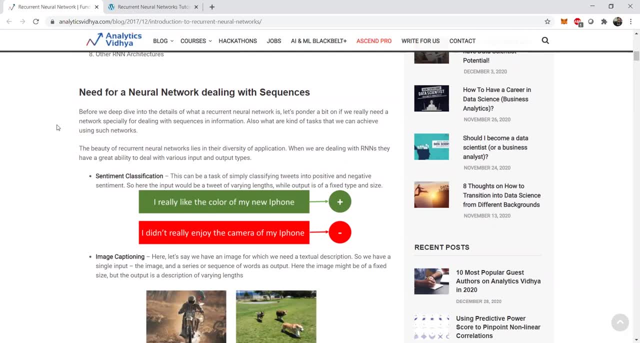 Now, why do we need recurrent neural networks? is because when we are talking about, particularly in the field of NLP, when we are talking about context of a particular sentence or a particular word in a sentence, Which is generally need to refer to what words or phrases are present, 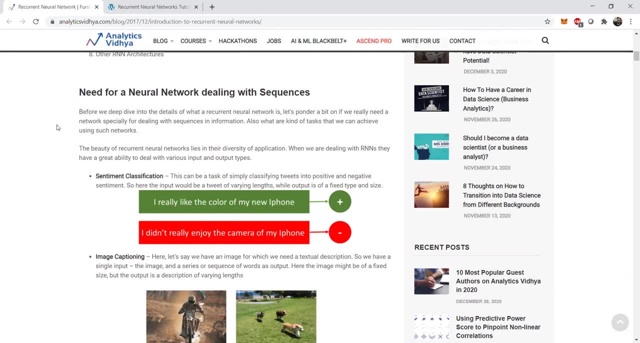 forward to that particular word and backward to that particular word. That means we want to capture the context of a particular sentence right And in that case our recurrent neural networks perform the best. They have this different activation units inside them. They have recurrence relations. 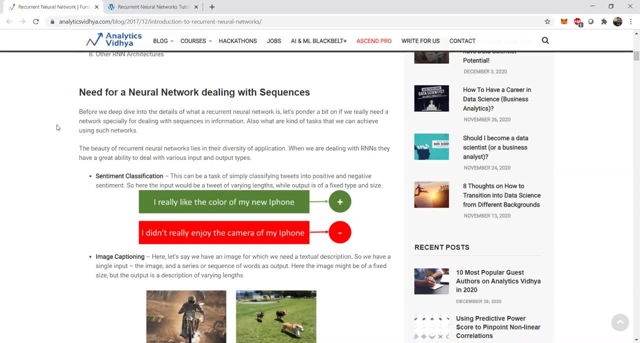 which allow different, based on certain time steps. they allow the memory to capture all the sufficient information required for a classifier, generic machine learning classifier or any NLP classifier- to perform its tasks. So sentiment classification is by far one of the most you know most. 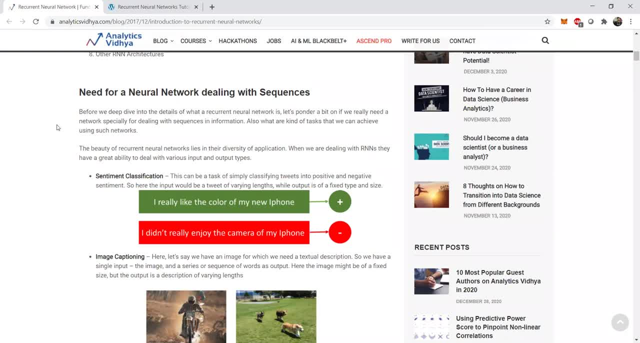 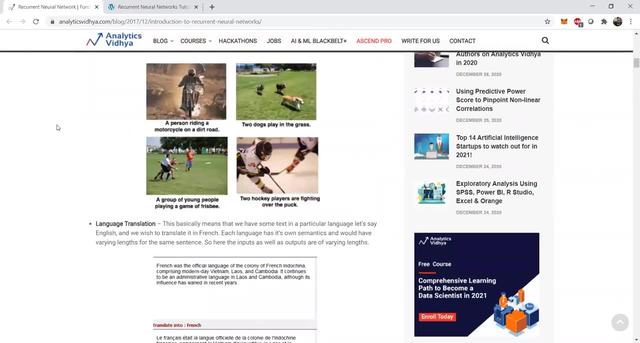 applicable genres of recurrent neural networks because they have been used extensively in this aspect And in other contexts. when we come to language translation, where we want to convert from one language to another language, let's say English to French or French or vice versa- we can. 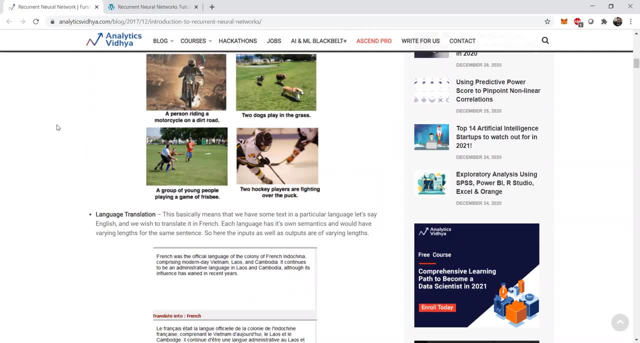 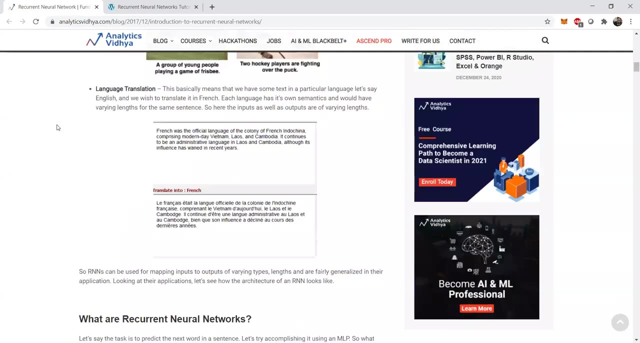 generally get to know more about recurrent neural networks and how they can optimize by understanding different contexts present in different languages and also analyze them. So in this example we see that there we have a French corpus and then correspondingly English corpus. So, with the help of RNNs and all the you know, sophisticated 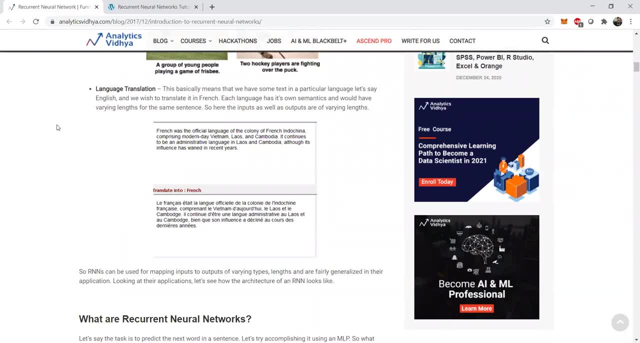 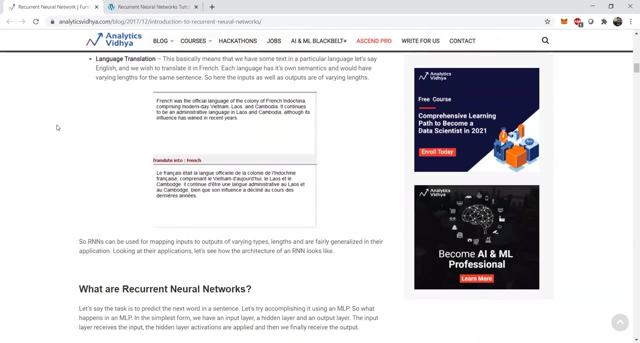 architectures which are currently in present, we can generally translate from one language to another And this has greatly enabled us to build a scalable and highly like having a very high throughput of RNNs. So RNNs are can be used for mapping inputs to outputs of various 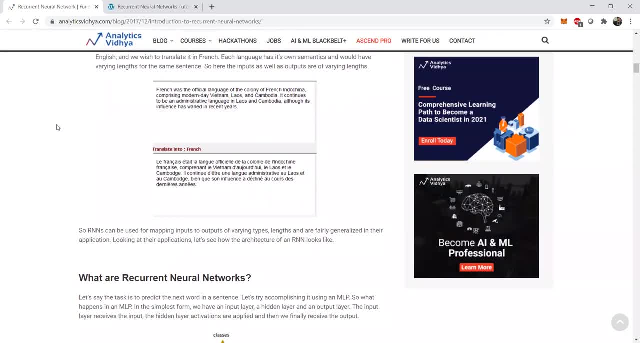 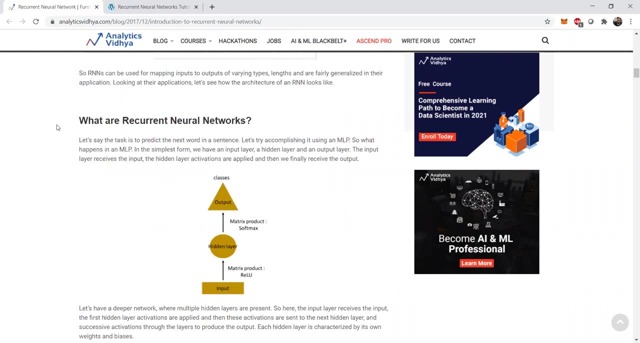 types, lengths and are fairly generalized in their application. So details of this: recurrent neural networks. Now, when we talk about recurrent neural networks we generally can think of it as a very sophisticated multilayered perceptron or a multi MLP in general. So what happens in? 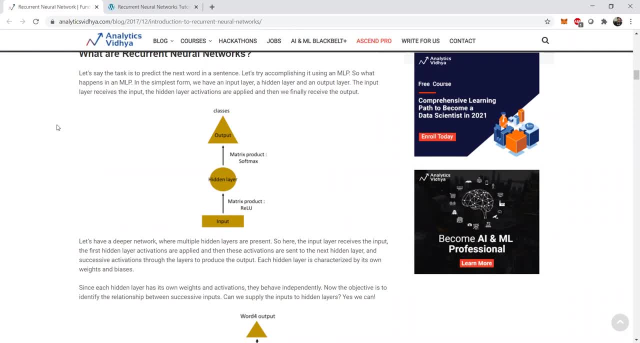 MLP is that we have an input which collects the input features and we apply some kind of nonlinear activation units on it, on that particular inputs, and we get the output of that, of those input features. And these nonlinear activation units can be anything ranging from sigmoid, softmax, ReLU and 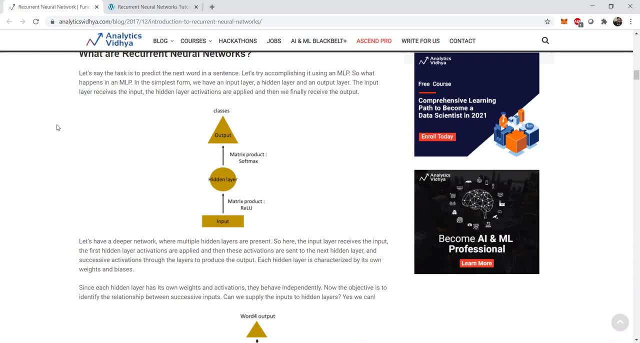 these kinds of activation units are present to allow some nonlinearity in the input features. Now, when we have a deep network, when we design a deep network, with just basic MLP, there is effectively no memory retention or there is effectively no- you know- memory present which can capture sufficient. 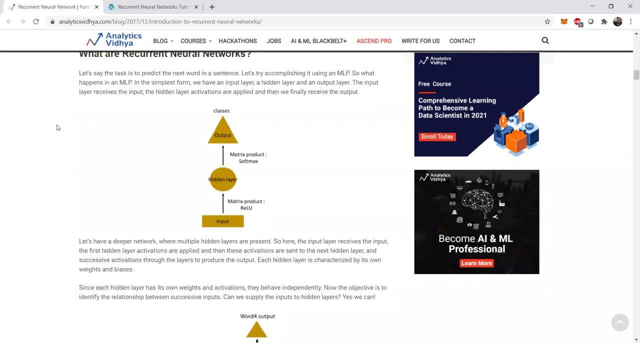 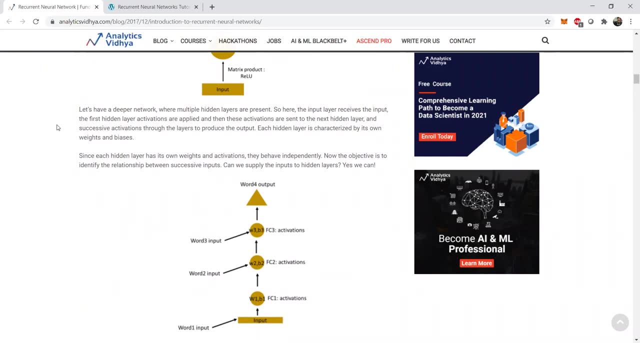 information from a particular text or a particular NLP corpus. So that is where the recurrent neural networks comes into the picture. Now, if we, if we were to unroll a recurrent neural network, we would be able to see that a classic diagram. 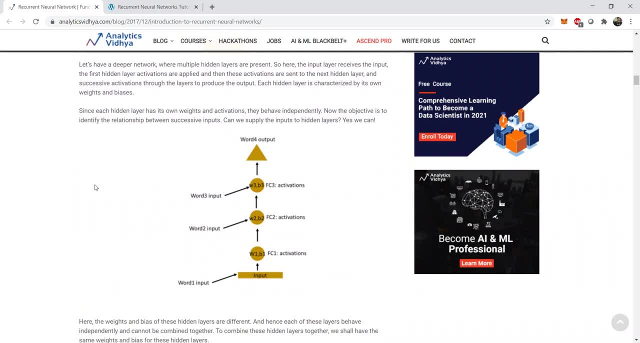 which is present here, word input right, and we apply certain activations in a series of steps, one after the other. So if we have a particular word, let's say word one, as the input an activation comes into the picture, which. 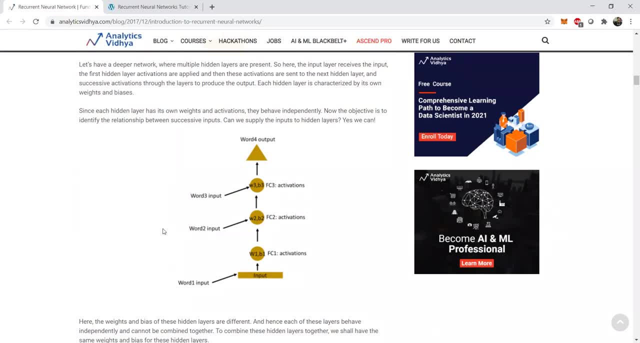 gets applied on W1, that is the word vector input And the output of that particular activated layer is the input to the next layer. So in this way there are lots of hidden layers in between in an unrolled recurrent neural networks. But 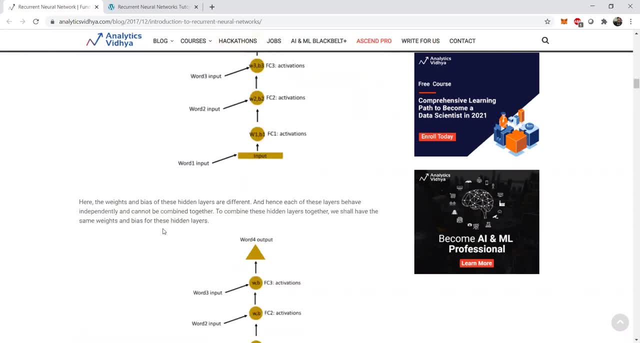 all these kinds of things often happen because we are unrolling a recurrent neural network. But if we were to design an RNN from scratch, we would be thinking them as similar to a recurrence function, which can be viewed in this example over here. you can see that we have an input. 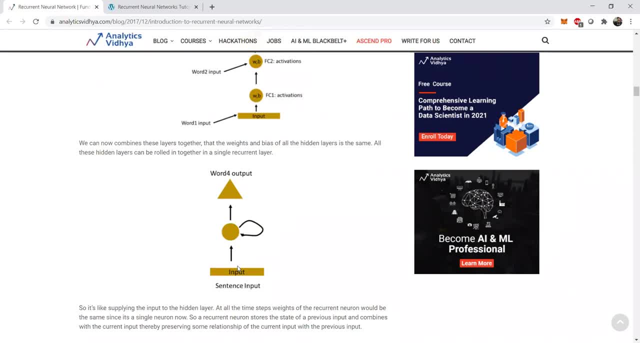 sentence or an input feature vector, and we are passing it to a hidden layer. Now that hidden layer has an arrow loop, which is which is, which is a self loop, And it is running back to itself. Again, this implies that the intermediate parts, that is, 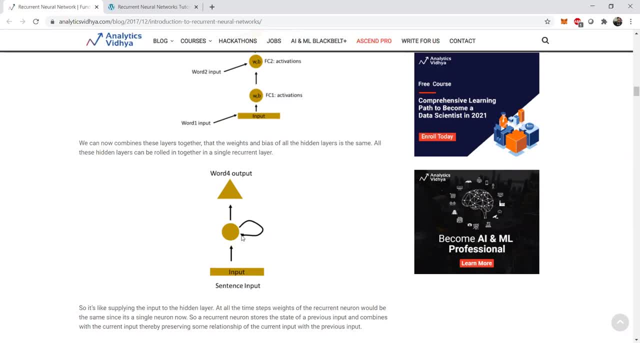 the intermediate, hidden layers of a recurrent neural networks are following some kind of recurrence. Now, recurrence is a general rule in computer science when we want to apply a function which which is almost as similar as which which ranges actually based on certain time. So, for instance, if time equal to t zero, the function has a value. 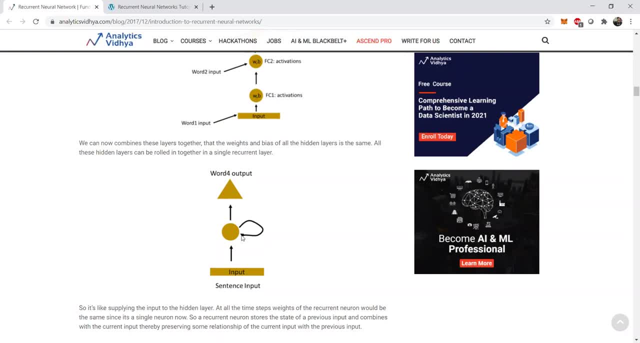 of n, the time equal to t one. you know that same function will take the value of n plus some added features. So the every, at every timestamp, some of the input features of the previous timestamp will be will be present as input features. So recurrent, neural. 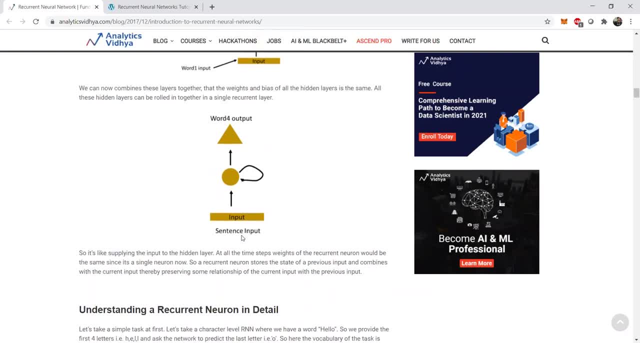 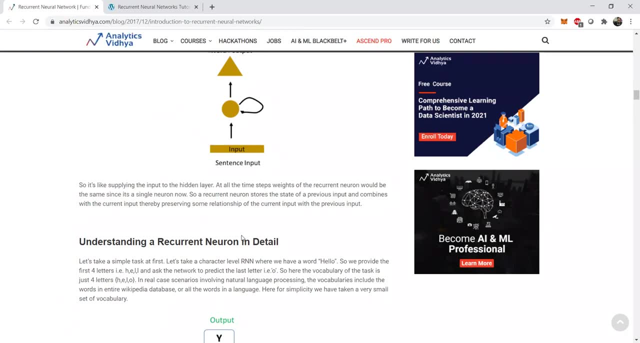 networks apply this concept only Now, if in a general, recurrent neural networks, since this is a neural network topic, there are two broadly different kinds of things which are happening. So one is a forward pass, which which computes the weights and the biases of the input features. And then, since this 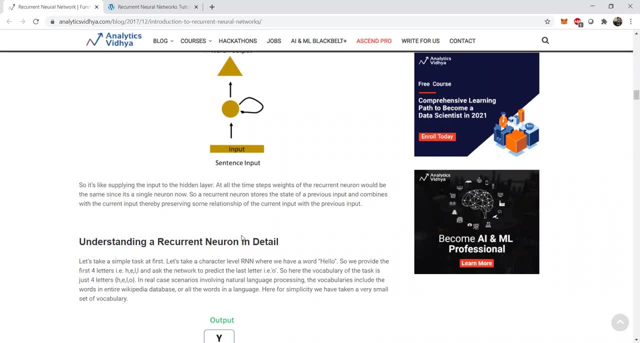 we are performing supervised learning, then we compute the entropy, then we compute the loss that we have- either a categorical loss or a binary loss. we compute the errors and we try to backpatch through the recurrent neural network, and this is where the performance enhancement comes. 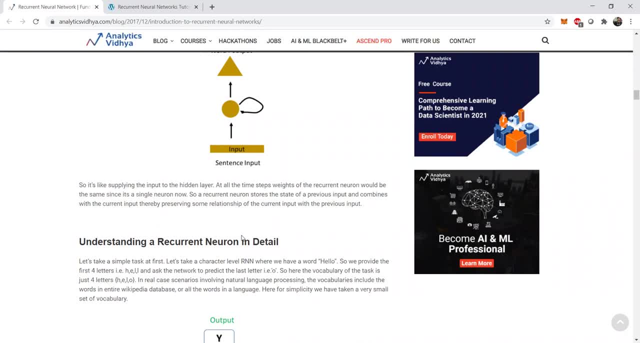 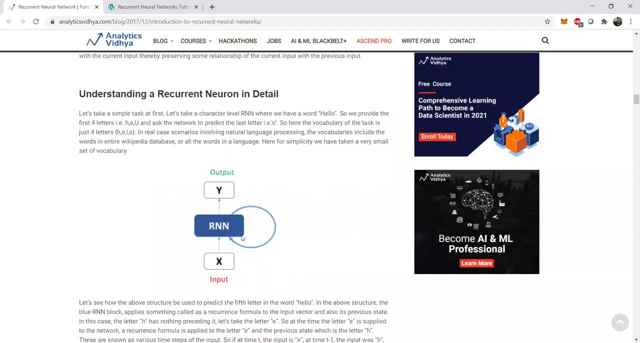 into the picture Now. in this case we will be talking about the forward pass in this, in this mechanism Now typically a recurrent neural network- in detail appears like this: You have an input feature which is x, and it passes through a recurrent neural network unit which is a self loop on it, and then it provides the output. 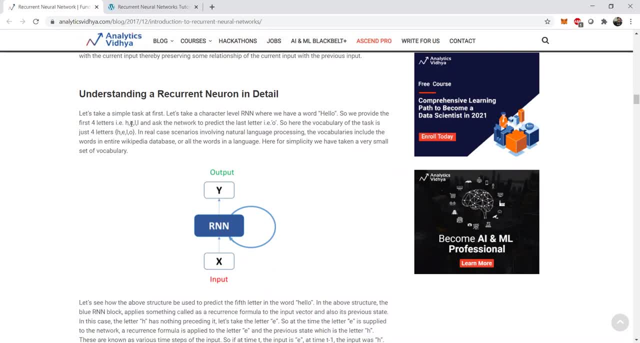 Now, in this case we have a four letter word, that is hello, The first four letters, that is hell, and we will ask the network, that is the RNN network in the forward pass, to predict what will be the next letter. So here the vocabulary of the task is just four letters, that is hell and o. 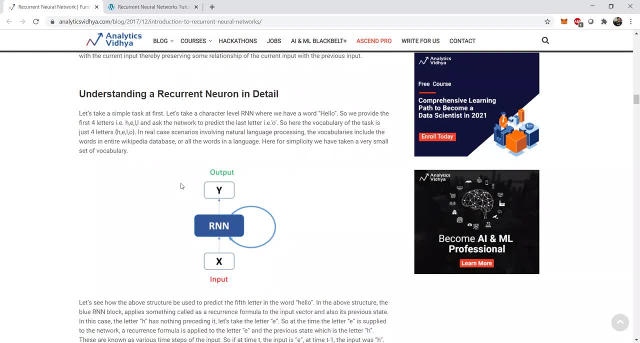 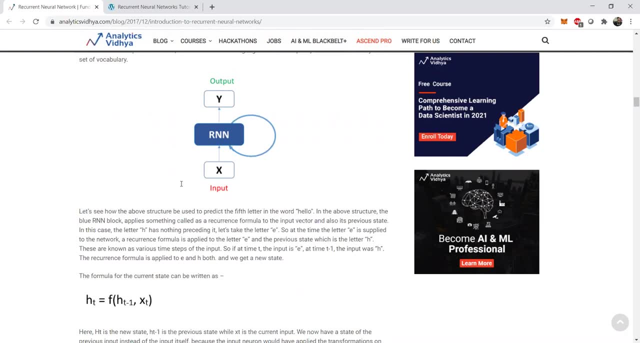 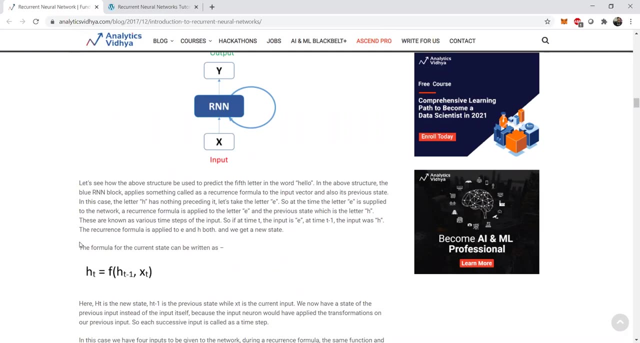 Now, in most of the language NLP situations, this prediction is what gets output. it becomes the output in a general classification tasks. Now if we were to design a particular RNN, so that would look pretty much similar to something like this: If we consider the hello example at time, step t, if we, if we just pass the first four letters. 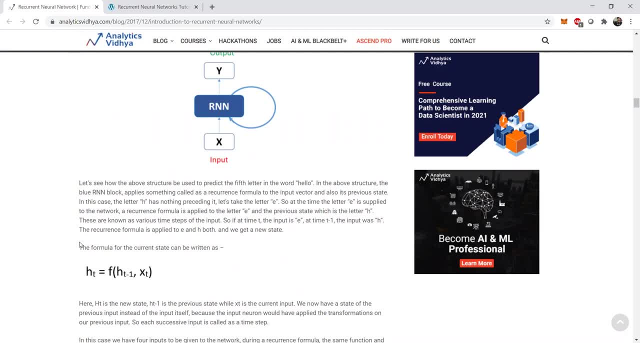 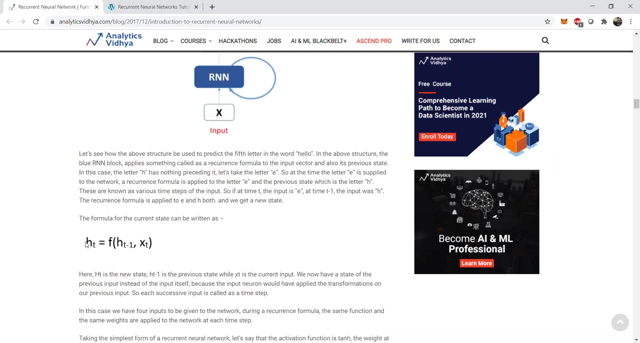 that is hell. then we in the time step t equal to one. that is the next time step. we will be passing ell and o. So at each time step we are just picking what will be the next character from it. So if we write this in a recurrence formula, it becomes ht equal to f of ht minus one comma. 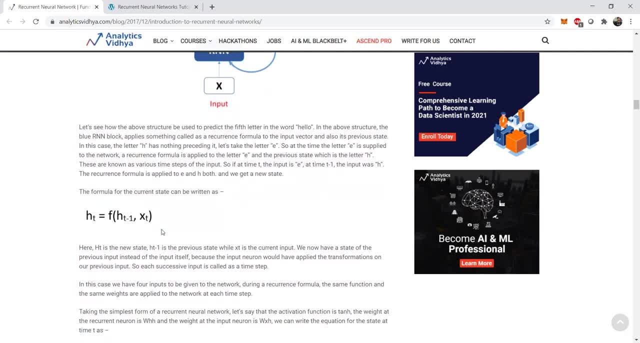 xt, Where ht is the new state And ht minus one is the previous state, while xt is the current input. Now we have a previous input instead of the input itself, because in recurrent neural networks the input neuron would have to be applied on the transformations of the previous input. 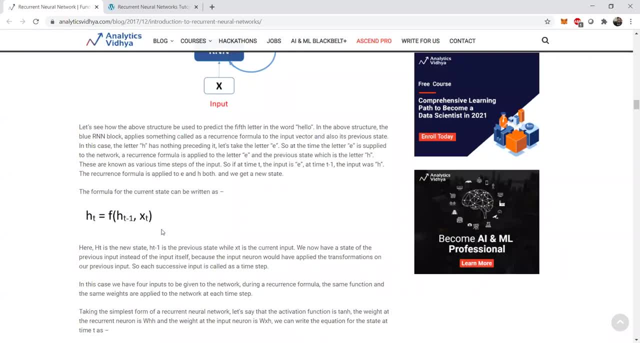 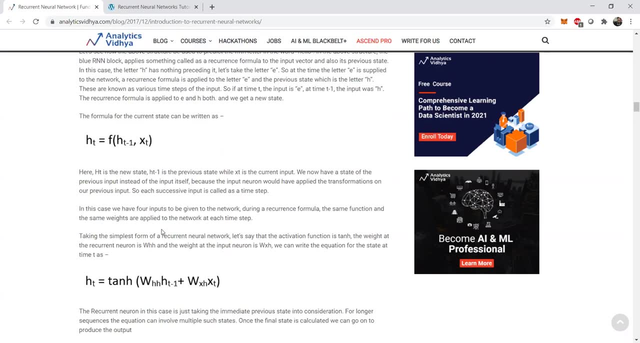 That means at the time step t equal to t1. what was the outcome is dependent on the time step t equal to t0. that was the previous outcome. So in this way the recurrent neural networks try to apply this in a sequential manner, In a sequential recurrence manner. 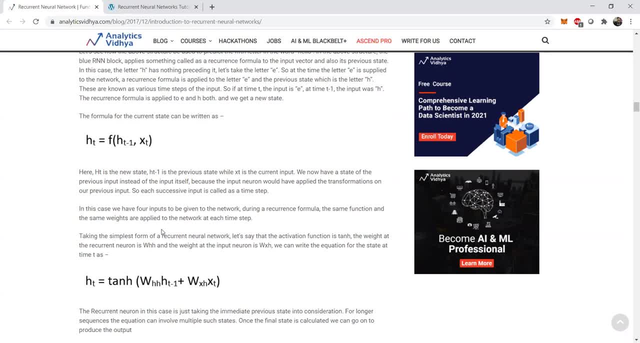 So if we were to take this simple example where we have ht equal to f of ht minus one comma xt, and we will be applying some kind of non-linear activation on it? Now, the design of this is very similar to what a multi-layered perceptron is. 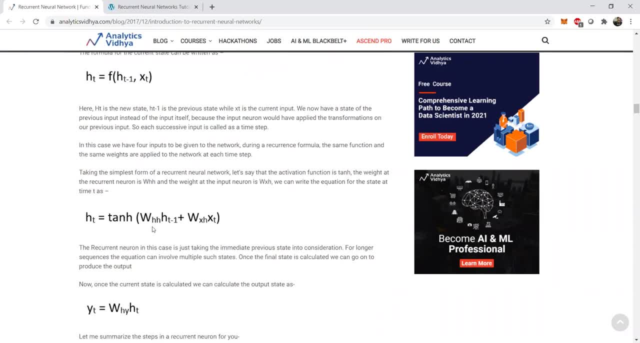 We are applying a linear activation which is given by this equation over here: ht equal to tan h. of this, this is a particular weight matrix that is given by w hh Times, the ht minus one plus w xh. this is another way to a weight matrix with xt. 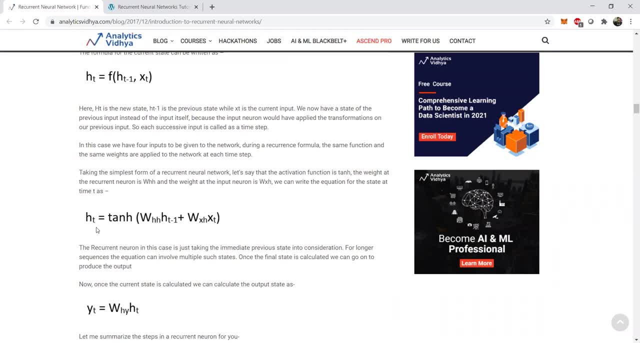 So effectively we get a coupled equation, having a non-linear activation unit called as tan h, and we are having some associated weights. the weights are associated with the ht minus one, that is the previous state, and also the xt, that is the input state. So we have two different kinds of weight vectors over here, the w hh and the w xh corresponding. 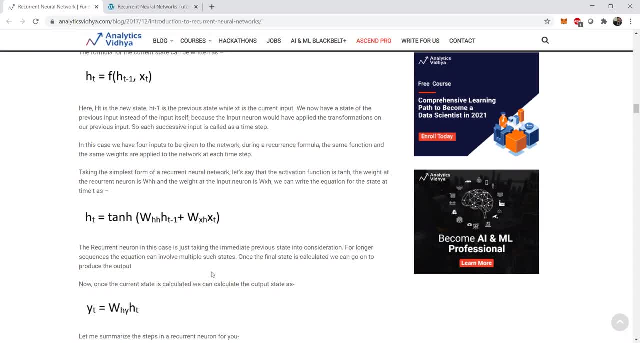 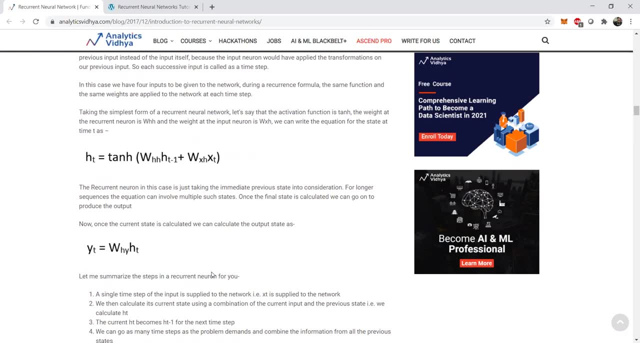 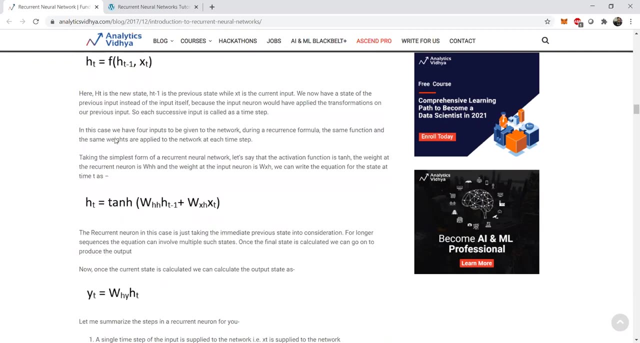 to the y, ht-1 and corresponding to xt respectively. Now this is the internal layer of a particular recurrent neural network. Now if you want to compute the output that is the y in our figure, this y in our figure, we have to just apply the output that is the ht. 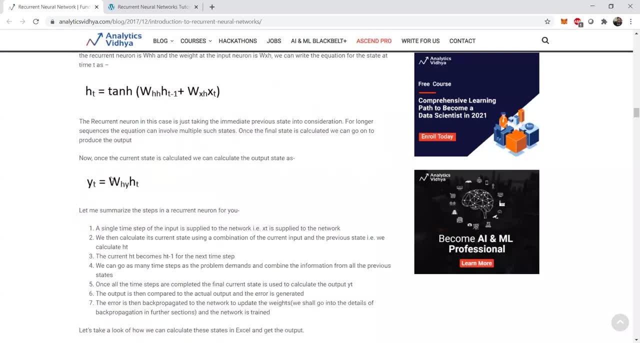 We have to apply some weight on it. So in many cases this is the most simplistic output where we apply a weight. that is why, on top of the output of the previous layer, that is ht, or we can apply a non-linear activation on this. So either it can be yt equal to some non-linear 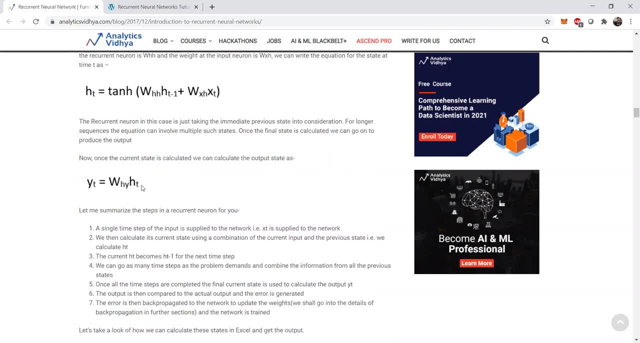 activation times this, why times ht? or it can be simply as: why times ht? So if we were to summarize this entire step of how recurrent neural networks work, So a single time step of the input is supplied to the network, that is, the input feature, which is, in our case, the 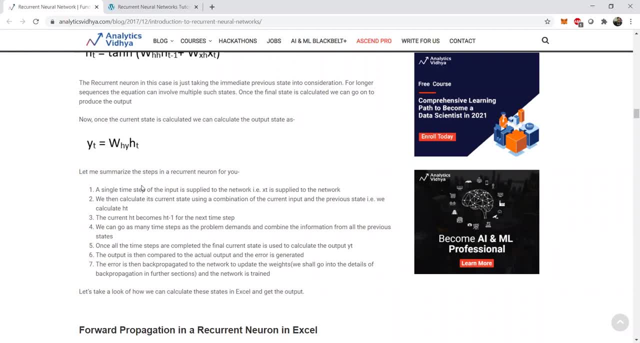 xt. We then calculate the current state using a combination of the input features: the current input and the previous state. In the previous state, if we have the first time state, then the previous step will be zero. So initially we calculate the ht. Now the current ht becomes ht-1 for the next time step. So this is how the recurrence. 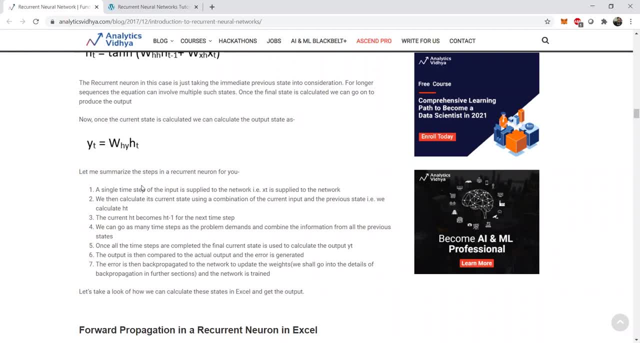 pattern is followed in recurrent neural networks and we can go as many time steps as we want, as our problems define that, and we can combine the information from all the previous states. So in this way we have a recurrent flow of inputs and recurrent flow of weights. 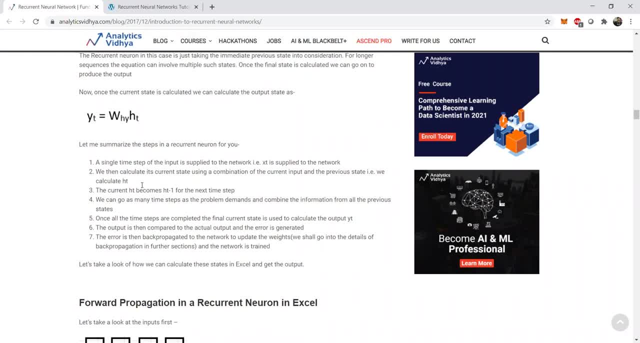 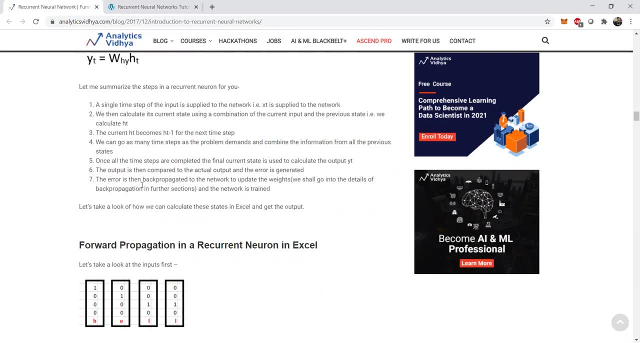 and biases at each step of the recurrent neural network. Now, once all the time steps are completed, the final current state gives us the yt. that is the output Now. the output is then compared with the- you know the predictor. that is the actual output, just as in the case of normal supervised. 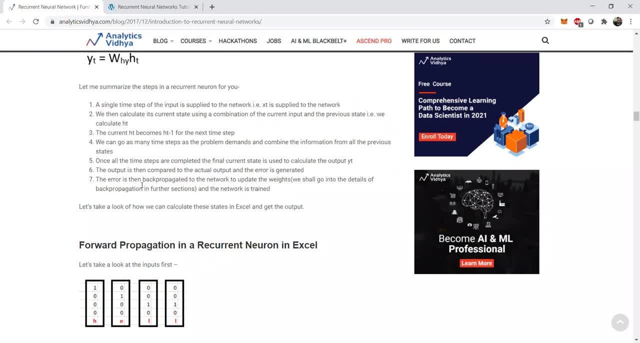 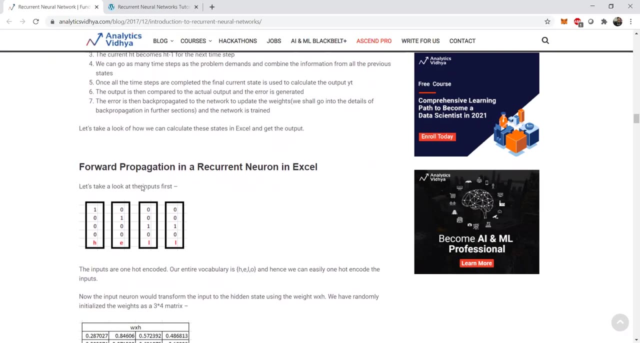 learning right. and then we can do the back propagation, to calculate, to change the weights, to update the weights, to make the difference or the error as small as possible. Now, in this case, let us take an example to see how the forward propagation, or generally referred to as the forward pass, takes place in an RNN. So in this, 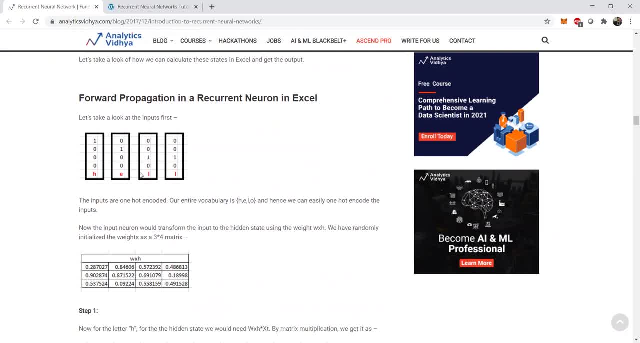 case, if we take the first four letters of the word hello, h-e-l-l. so we see that this is a, you know, a tensor right having zeros and ones. Effectively, this is known as a one-hot encoded tensor right, and in this case you can also get to know the dimensions of this. So it has only 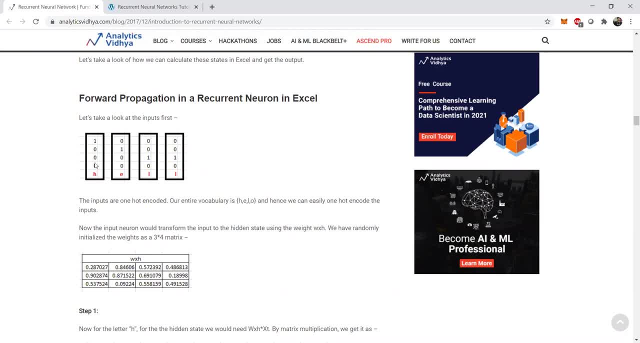 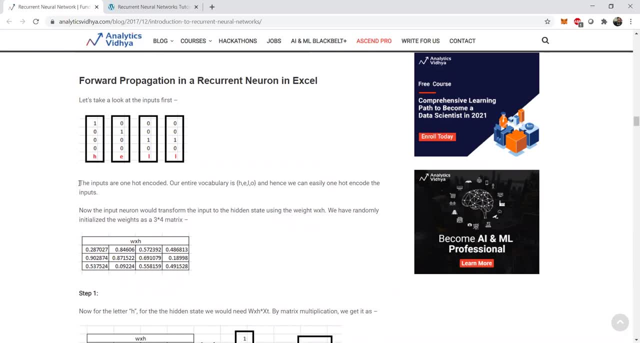 one column and four different rows pertaining to the ones and zeros which are present in it. Now, one-hot encoded vectors are effectively very. they give very sparse matrices or very sparse tensors, because only one element is one and the rest, all the elements, are zero. And let us now 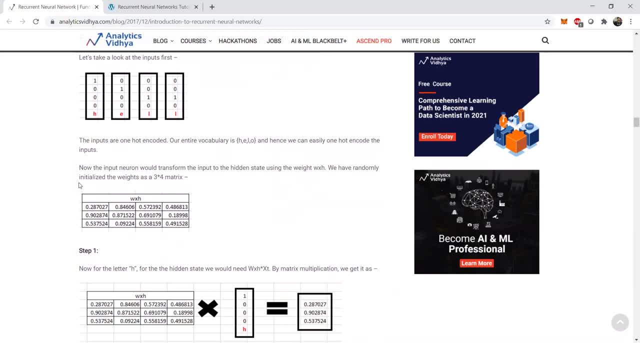 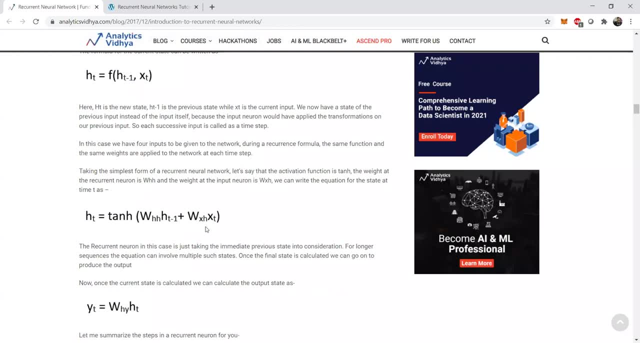 initialize our two weights, that is, w-h-h and w-x-h. If we remember in our equation that we have we have two weights: one is w-h-h and one is w-h-h. Now we have to initialize those weights. Now let us initialize them randomly, as it is done over. 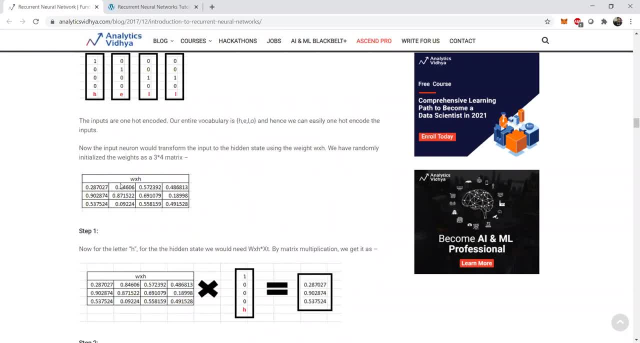 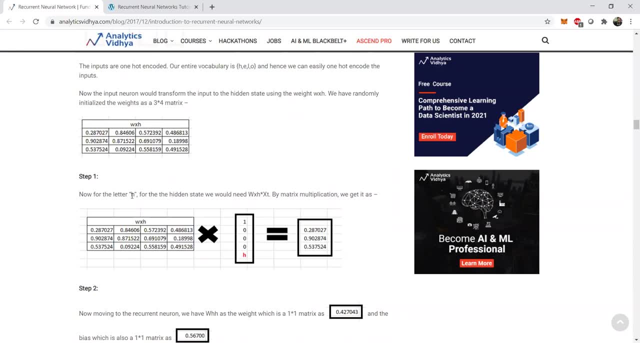 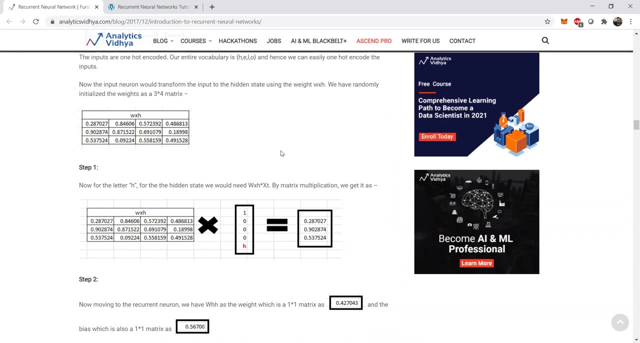 here. So w-x-h is defined by this tensor having these weights corresponding to h-e-l-n-l right, and then we have for the letter h and for the hidden state we also need w-x-h right. So by matrix multiplication, which is given by this equation, w-x-h into x-t, we get. 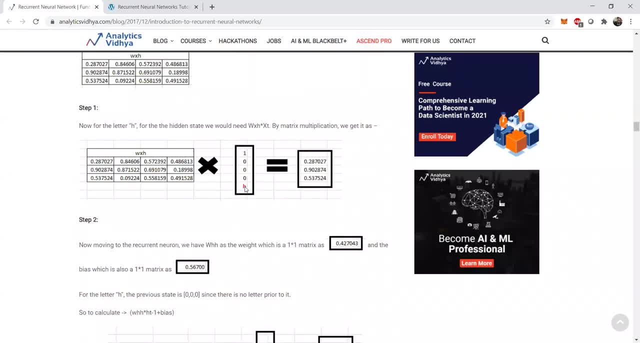 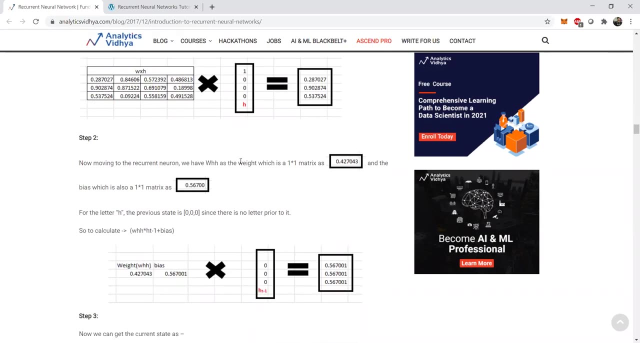 we multiply w-x-h into this h, that is the first letter, and we get this as the output, this decimal values or this decimal tensor, as the output. Now, this completes the first step, where we have calculated the forward pass for h. Now, if we move to the recurrent network or the recurrent neural network, 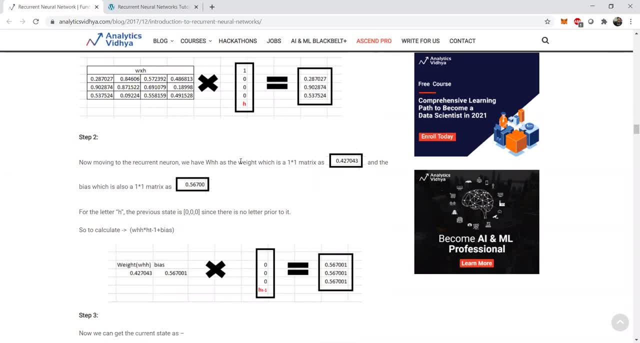 we also have to calculate the w-h-h, which is another one cross, one matrix. Now we have to take some bias. now it is recommended to take some bias, since most of the cases will be equals to zero, but for our case we, if we remove the bias, then our recurrent neural network 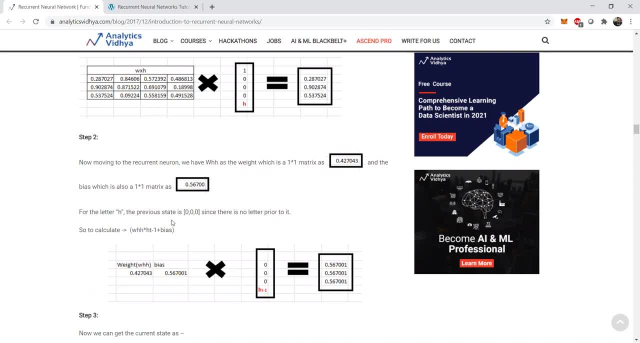 for the first step will only output zeros. why this will be is as follows: because for the letter h, the previous state is 0, 0, 0 because h is our first letter. and if and for the first letter, the previous state, that is the t minus one state, is effectively zero because h is our first state, that is the 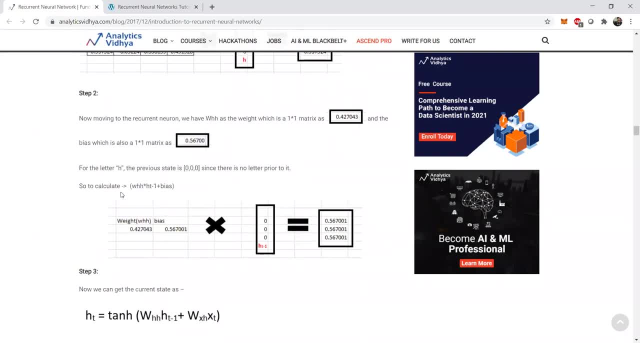 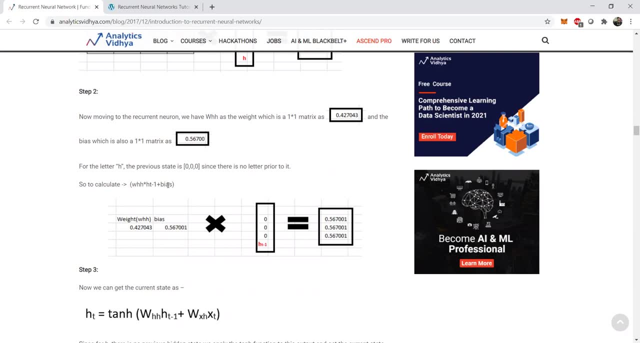 t equal to one. so for t equal to zero, the effectively the everything will be zero. So when we calculate the weights, that is, the w-h-h into h-t minus one is biased. effectively this part w h h into h t minus one, we are effectively multiplying. 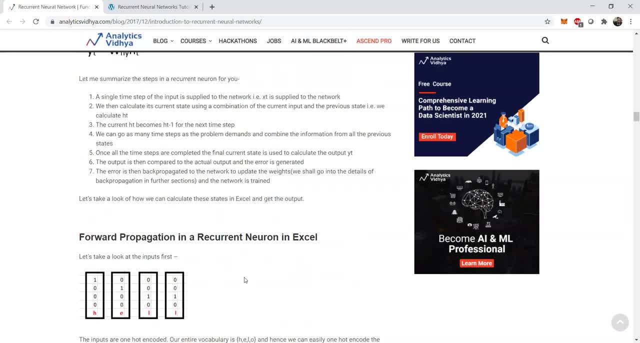 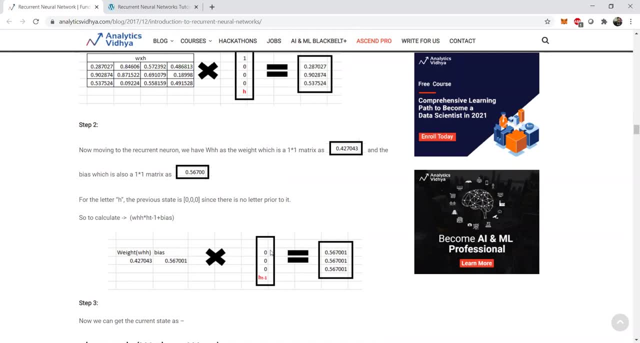 this um, this tensor that is 0.427, multiplied with this tensor that is h t minus one, because h t minus one is zero, the w h h into h t minus one also becomes zero. effectively, what we are, what we are left with, is just the bias. so if we keep our bias as zero, we can get to know that, you know. 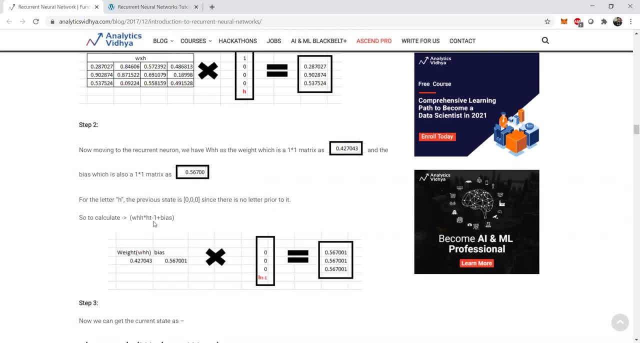 for the first step, everything will be zero. this particular part, that is, w, h, h into h, t minus one, this part will effectively be zero. so the output of the first one will be zero. but if we were to keep some bias- in this case we have a bias as 0.567, so that bias will get added with zero to. 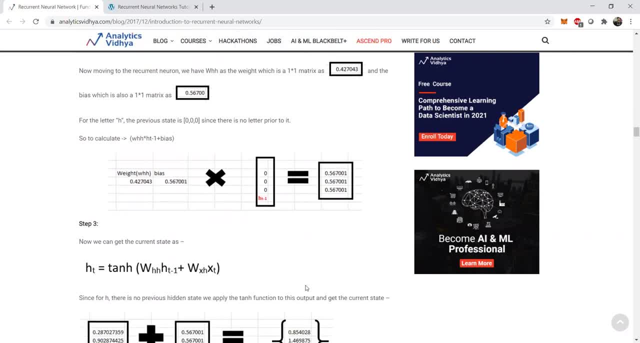 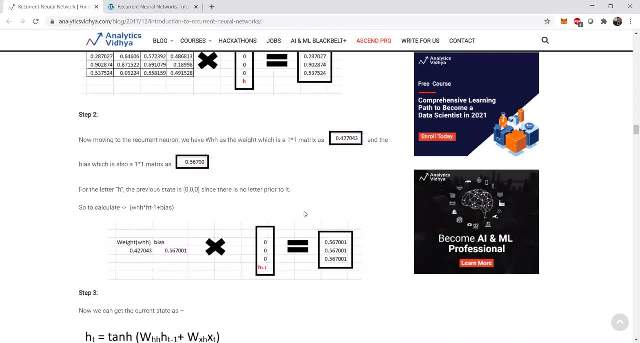 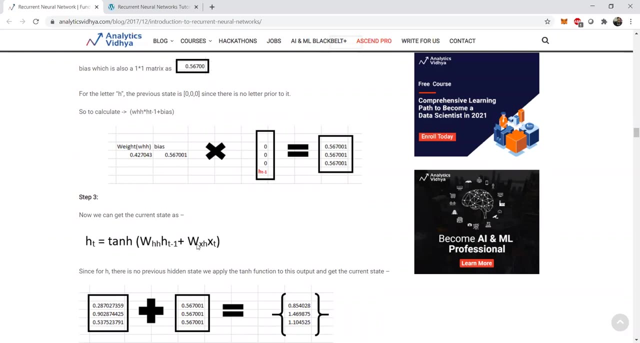 give some initial values, that is 0.567. now the step three is we have to add these two um. you know outcomes of these two um mathematical equations. that is, this part, this tensor over here and this tensor over here, because we have computed w h h into h t minus one, and we have also computed w x h into x t. 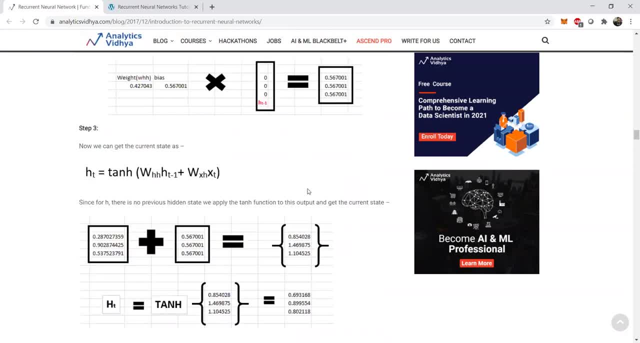 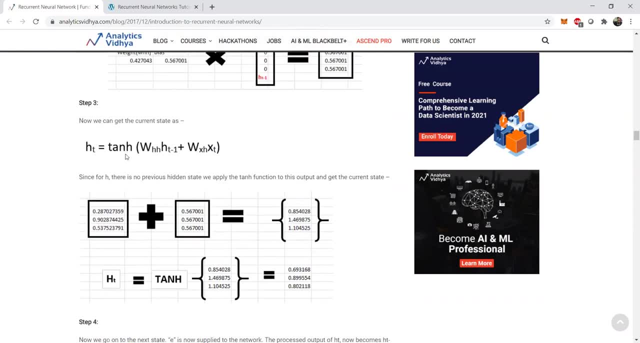 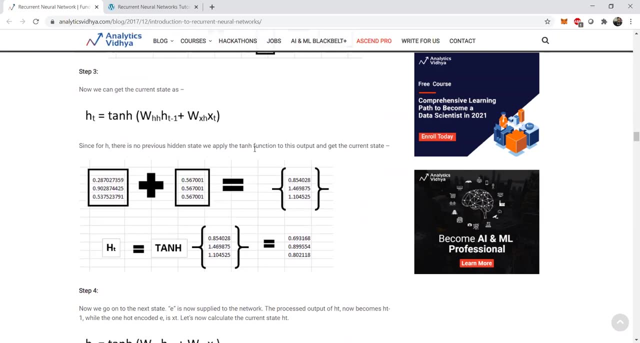 right and now we have to add them, which gives us these tensor of values, these floating point numbers, and then we have to take some non-linear activation on it. in general, in record and neural networks we are mostly concerned with tan h, because tan h has some important properties of. 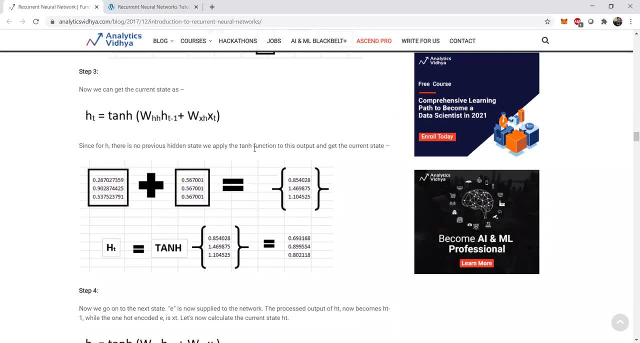 memory restoration and memory and capturing a lot of memory information from textual corpuses. that is why tan h is mostly suitable. and there is another mathematical importance of tan h because the second derivative of tan h dies down very slowly. now, if we were to do a derivative of tan h, 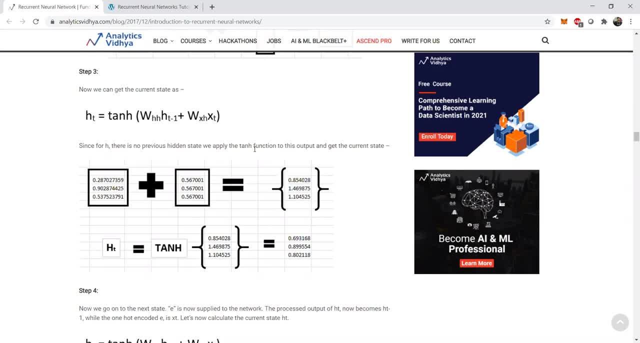 of a function x, the first derivative would give you one minus x squared. and if you were to do the second derivative, the second derivative will not. will would not be, you know, extinguished at a very faster rate. and that is where you know the tan h can attain or hold information for a longer time. 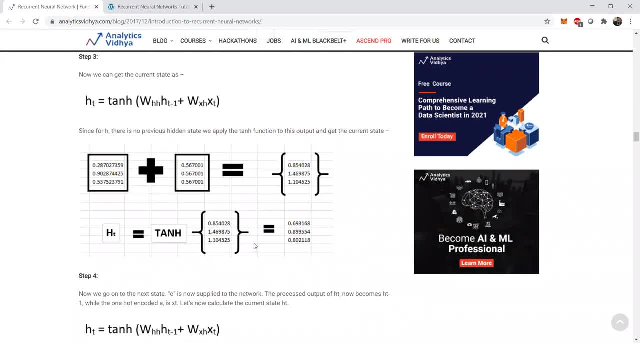 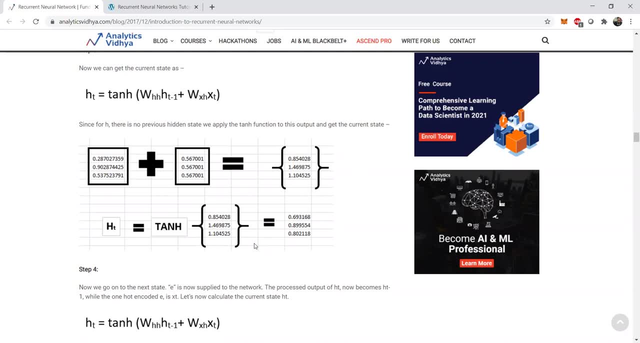 period as compared to other activation units. now, tan h has almost similar features and looks similar to a sigmoid function. it is almost. it almost has a kind of a shape curve. but it has different limits and different bounds as compared to sigmoid and that is why tan h is more. 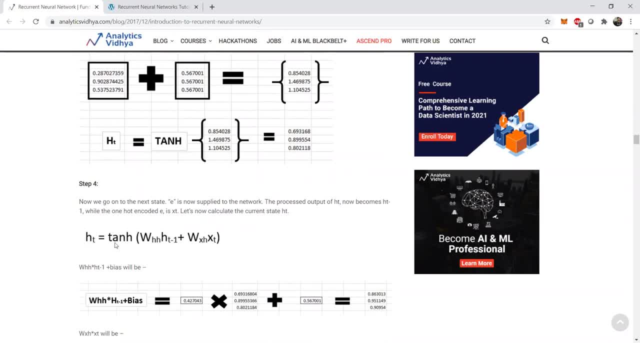 appropriately used. and the step four is: we have calculated the h t by passing it, the output of these internal mathematical equations through the tan h activation unit. now the next step is to compute the y t. now, if we were to compute the y t, the y t is is pretty much. 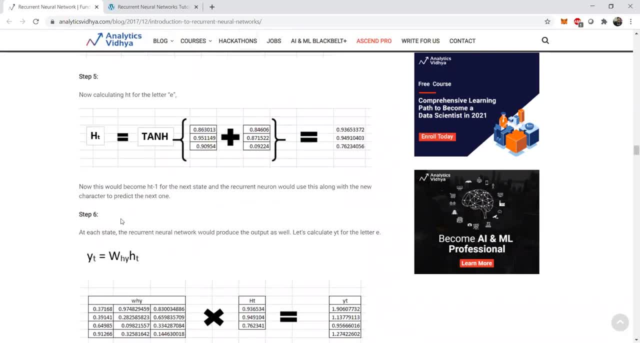 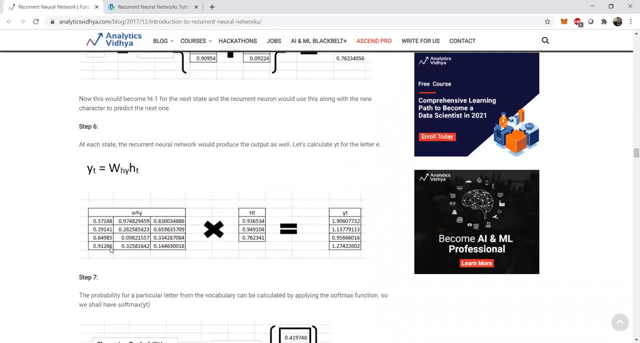 very, very simple, because we just have to multiply a weight, that is the h y. w h y multiplied, that is with the h t, now w h y is effectively the weight. that is uh. you can either initialize randomly, which is in our case, um, this has been initialized randomly, or we can initiate initialize them using: 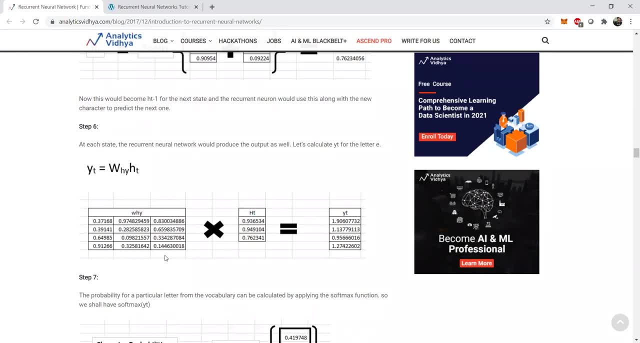 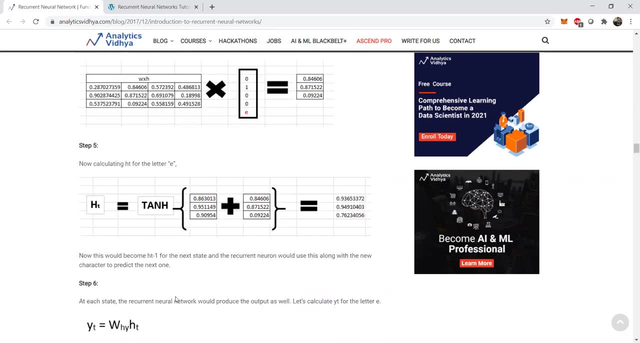 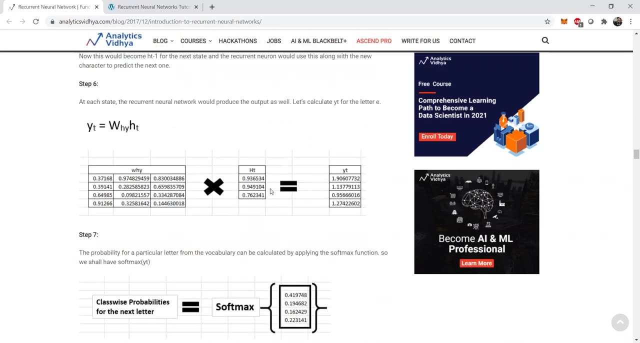 some activation units using some predefined formulas, or you can initialize them as zeros or ones, anything can be done- and we multiply it with the h- t that we have received from the previous step in our case. so this gives you the output of the entire recurrent neural networks for a particular timestamp, t. so we can see that. 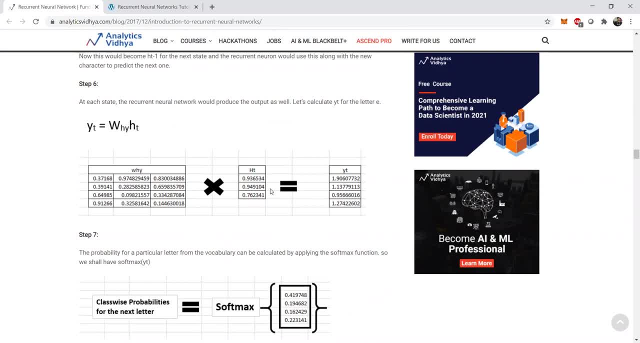 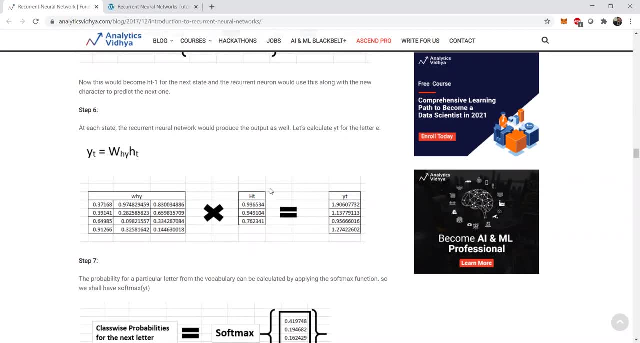 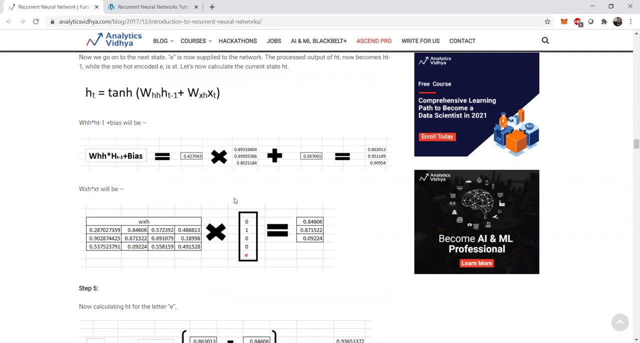 for particular timestamps: t. we can effectively uh take the information from t minus one and we are can also predict what will be the output or the next character in a particular sequence. now this uh, steps four and five, gives you an illustration of how you know the uh, how the next step becomes into the picture if you are taking 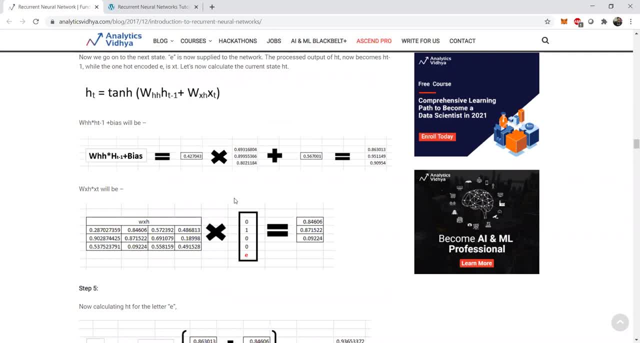 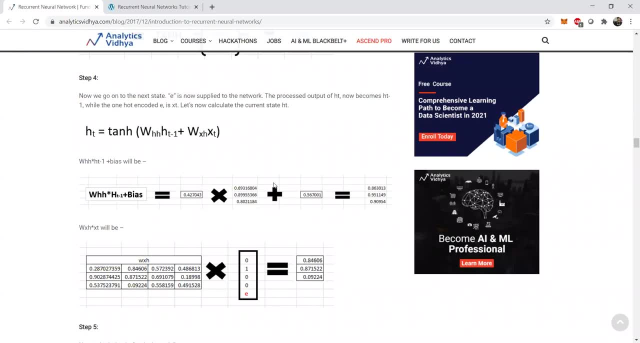 the next letter, that is, e, after h. we can also see that in the computation of the word or the letter e, we are taking into consideration the details that we have covered while calculating the values for h. so in this case, for each individual character, we are evaluating the characters. 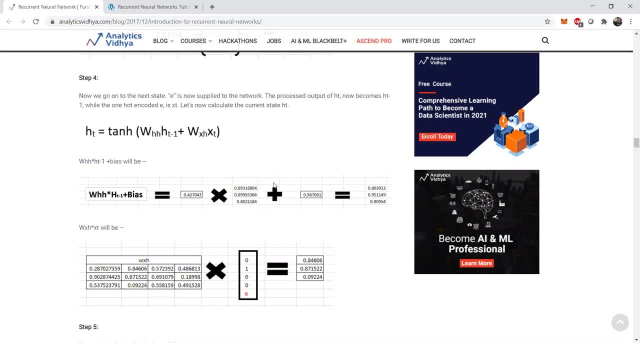 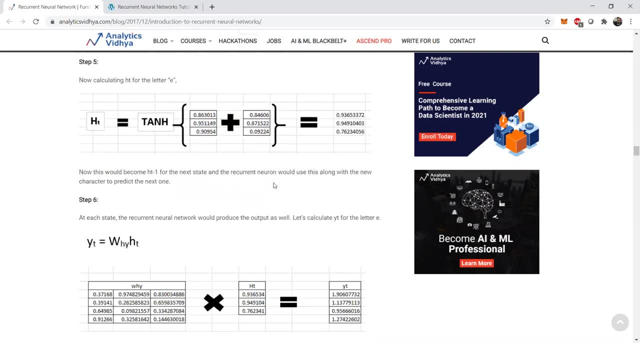 the details and the computations done on the character just before it and also for all the time, starting from zero. so in this way recurrent neural networks try to build a kind of a- you know- sequential network where you are calculating a particular output at a particular timestamp- t equal to t1- based on a certain previous timestamp, that is, t equal to t minus one. 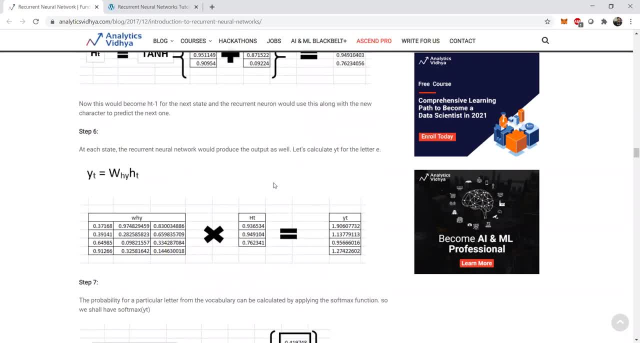 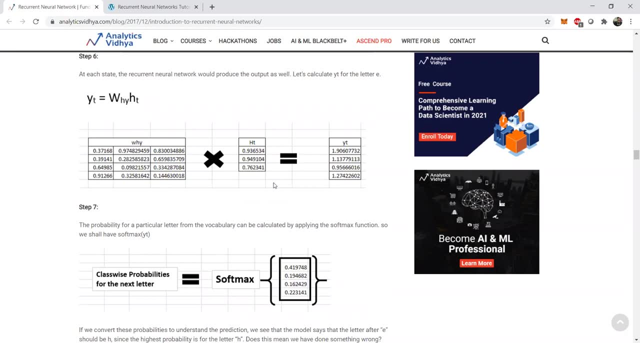 that is one timestamp before. so in this way the forward pass gets calculated. now, if you were to build uh, uh, we, when we get the yt, we effectively get us a series of probabilistic values. we get a t or a tensor of decimal values. now, if you want to apply some sort of classification context on it, 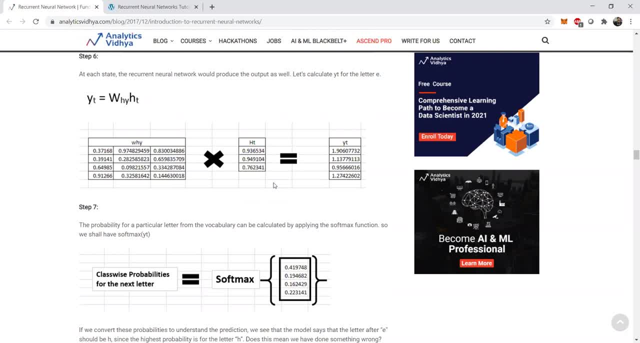 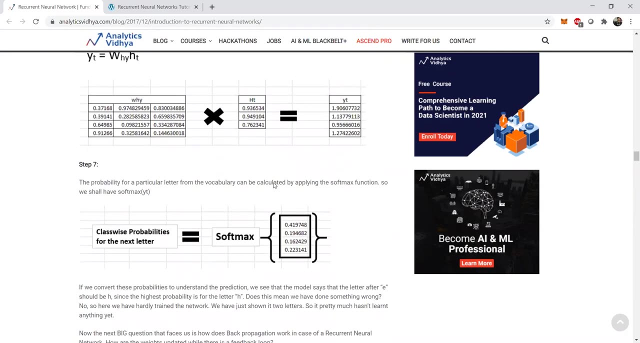 we generally refer to some activation units on those or an activation function on those output labels. now that becomes in most of the cases in rns. we use softmax function for that, where we transform the yt to a softmax variant or a softmax transform the output and this gives you a classified 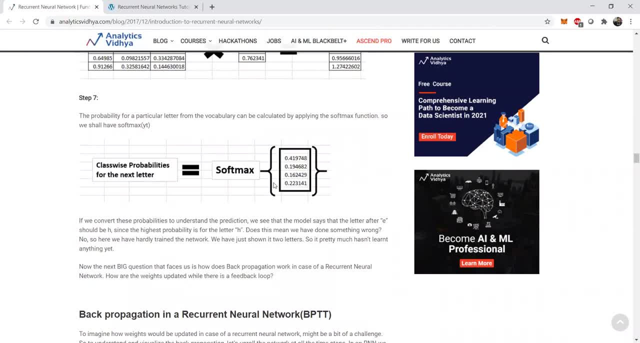 uh, probabilistic values where you can have certain values like 0.5- anything above 0.5 gets classified as well, 1 or anything below 0.5 gets classified as 0. so in this case you can have probabilistic values of. 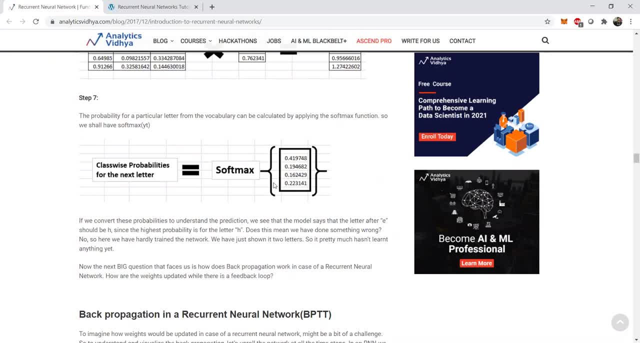 what the output. so this can also be used for predicting what will be the next character given a particular input character. so let's say, in the word hello- we have seen that hell is written- what will be the next character that will press? that will succeed l. that is the last step. so in most 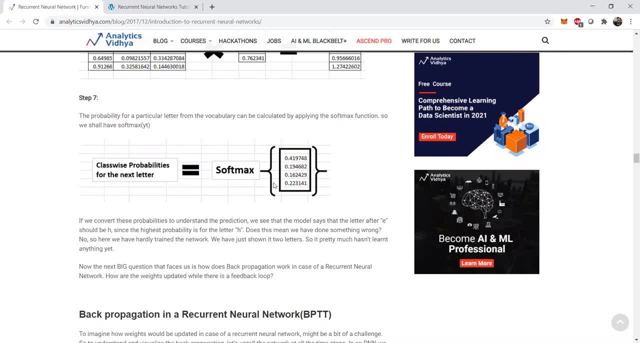 of the cases, after sufficient training, we will be seeing that oh, the, the particular character o, will will succeed l. so in this way, using this softmax activation at the output, that is, softmax of yt, we can effectively get all the range of probabilities for the from the, which gives you the most probable. 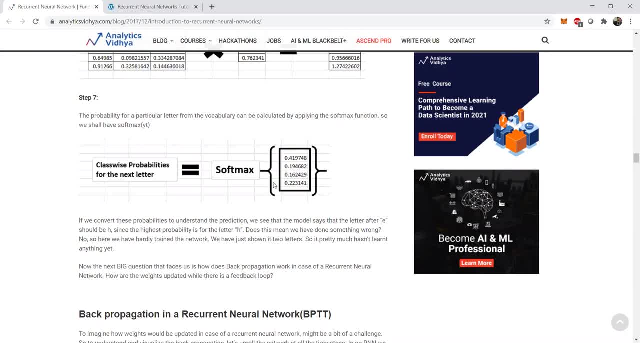 word next, next character and the least probable next character, and we can generally use this, uh, this thing, as a classifier, or or you can use this as a generative, recurrent neural networks. in this context, we have given the example of uh character level rns, we, where do we have? where we? 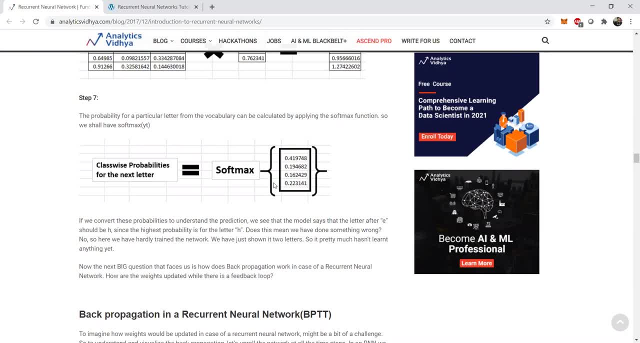 are applying this rnn concept recording neural network concept uh on particular characters in a particular word, but the same concept can be used in the case of uh words as well, you know. and next concept, since this part is generally considered as a forward pass of the first step, 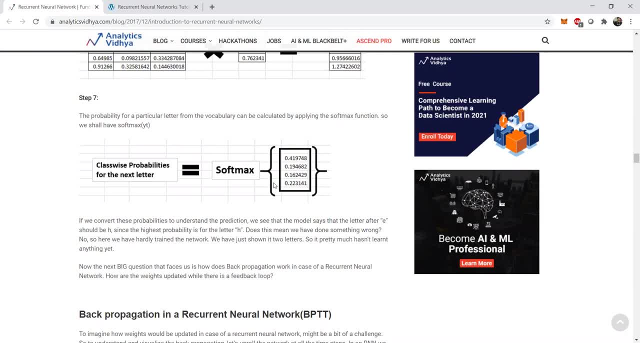 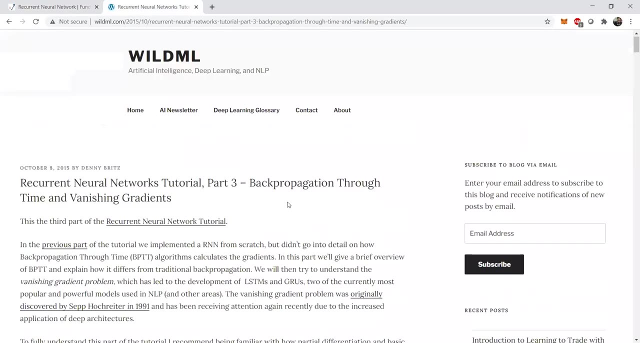 next part, we will be going towards the back propagation. for this back propagation we will be moving towards the next tutorial, where this is given in wi uh dwi rtm intelligence blog. so this is given really well over here by denny britts. so in this case we 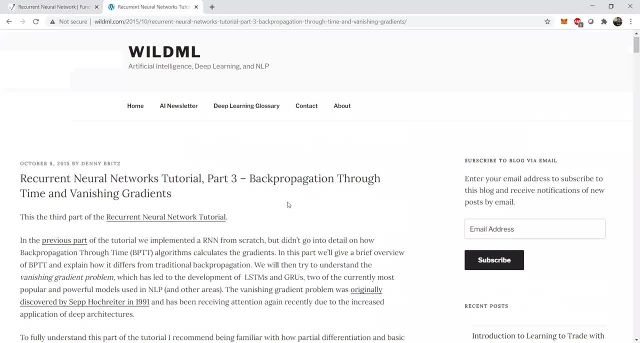 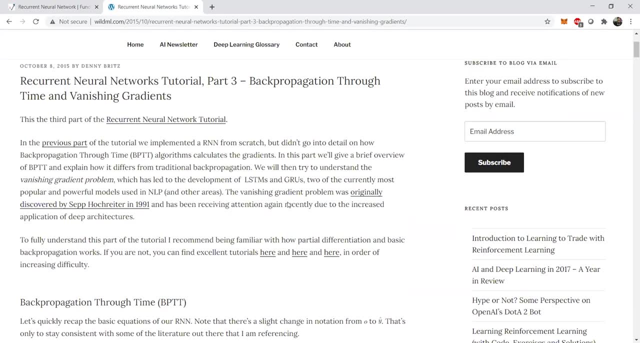 will be seeing how back propagation takes place now. we mentioned that neural networks generally have two kinds of passes. one is called the forward pass and one is the backward pass. now, the backward pass generally takes place due to the fact that we want the errors to be reduced. 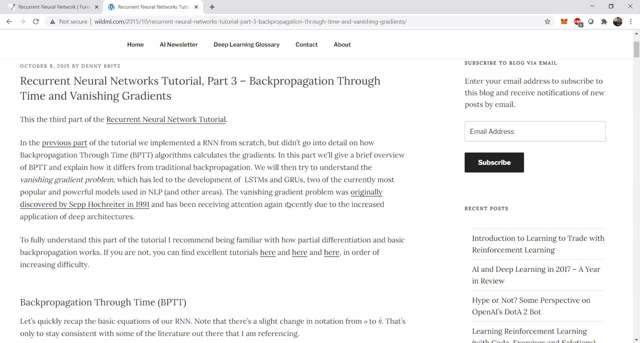 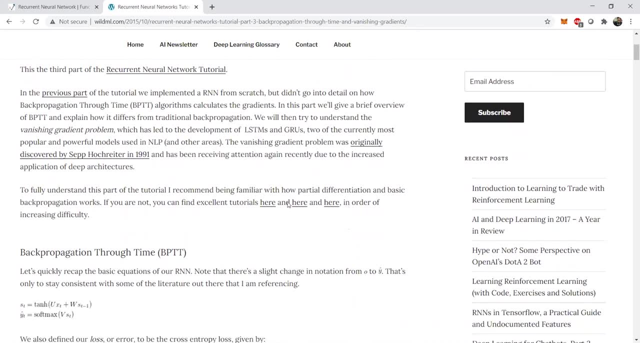 and we want, uh, very clear and crystal outputs which are almost very similar to the actual or the predicted output, predicted labels in most classification contexts. so in this case, since we have a time, uh, time space in consideration, so we can also consider- we can also label this as back propagation through time. 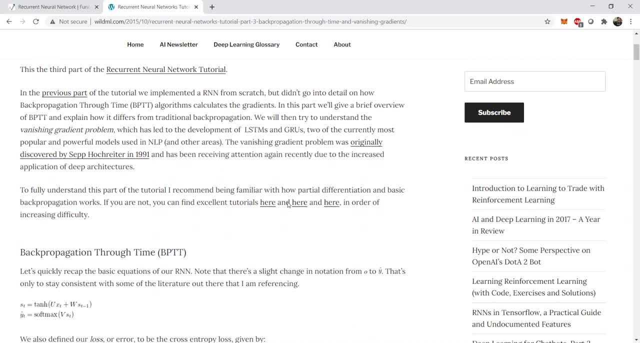 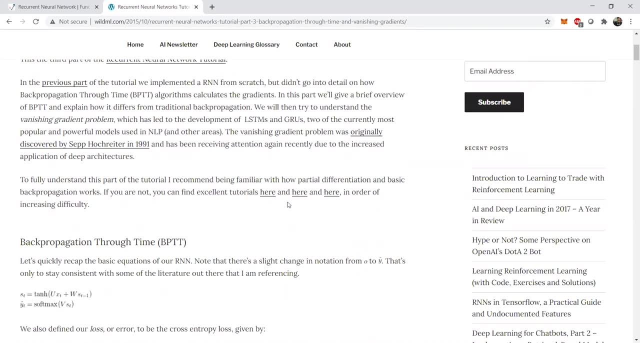 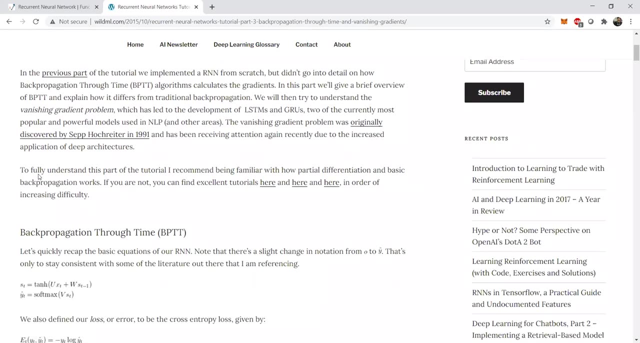 because we'll be seeing how recurrent neural networks actually actually apply gradient descent and gradient flow through time, uh, which was not in the case of normal multi-layered perceptron or dense networks. so if we, if we recollect, we can see that, uh, this is a variant of the same equation. 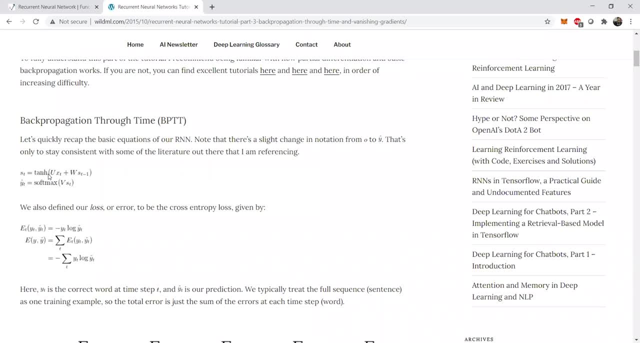 that we saw where we have uh tan h of the input features, w h h into h t, minus one plus x t into w a x h and then we apply um, a soft max of the output. if we, if we recollect in the previous block which we have we have seen now we can also define our loss. so our loss can be binary loss. 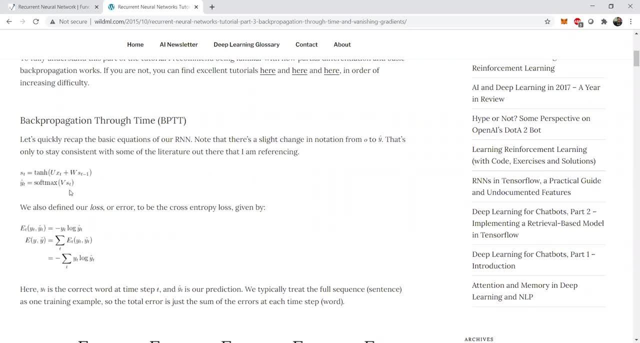 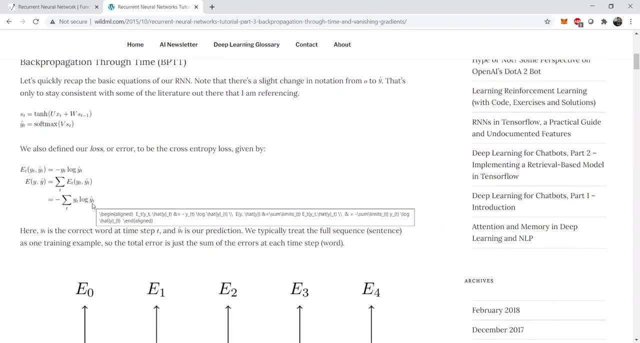 or it can be categorical loss. so if we, if we just consider our cross entropy loss, that is uh, we can just frame it as a very simple equation that is given by summation of y t into log of y t, y cap t, where y cap t is the softmax activated variant of the. 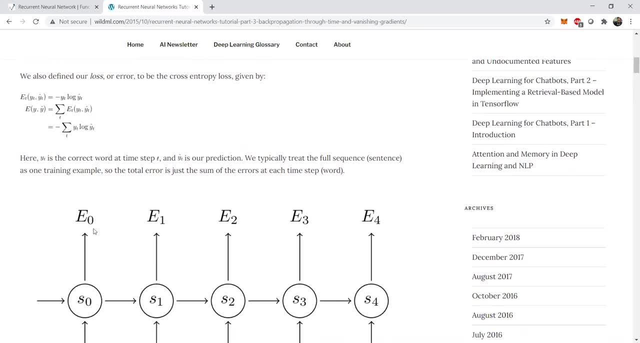 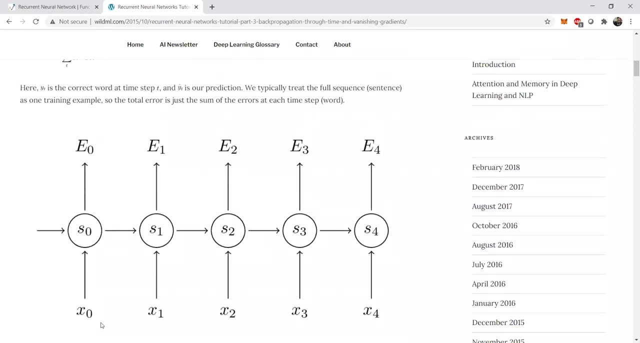 output: rnn- output in the forward pass, now typically an rnn like this. so, uh, zero for the s0 input. you have e0 as the output, x0 as the equal, and this gets forwarded to s1, which takes us input. the s0, that is the previous timestamp, right, and it takes x1, that is the input at the current step. 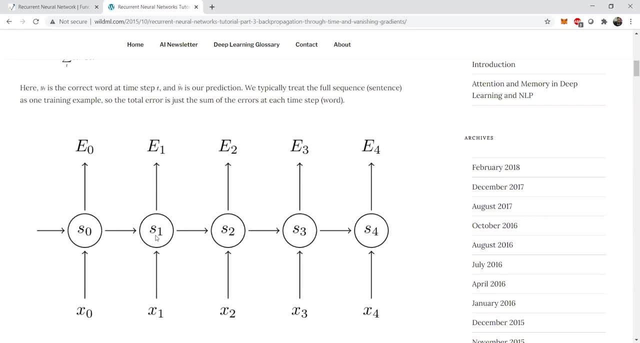 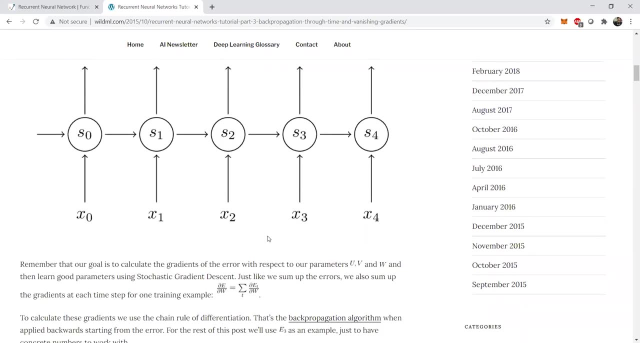 and it also gives you an output for the current step and it also gives you an output for the end step, that is e1 and is, and a part of the output is also fed to the next layer, that is the x, s2, and this is how the rnn takes place. now, if we were to consider the back propagation over here, 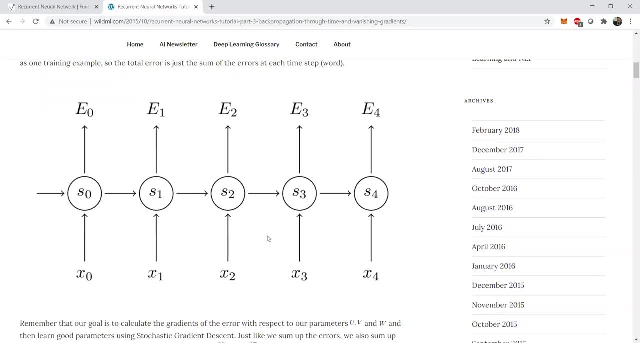 we want to do something called as chain rule differentiation. now, chain rule differentiation is the intuition for using. differentiation is because, generally, we are trying to optimize. generally we are trying to optimize a curve in a high dimensional plane by finding the minimum. now, why do we need the minima? because 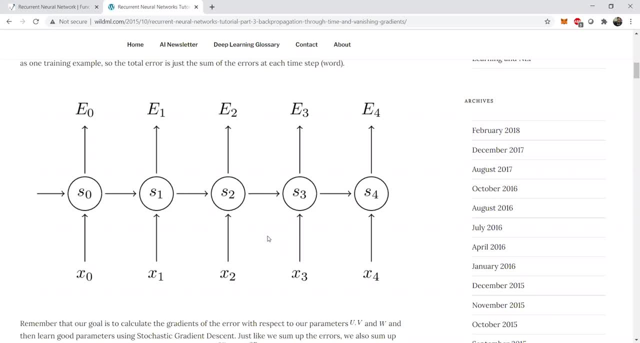 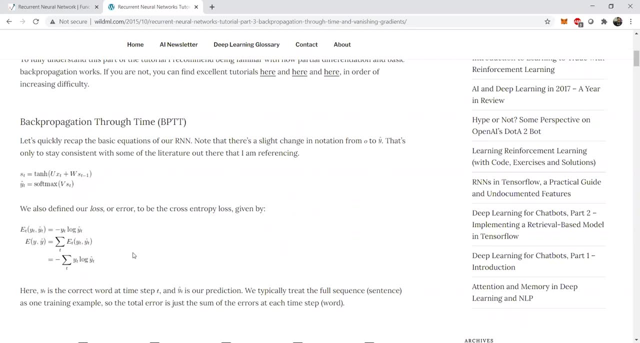 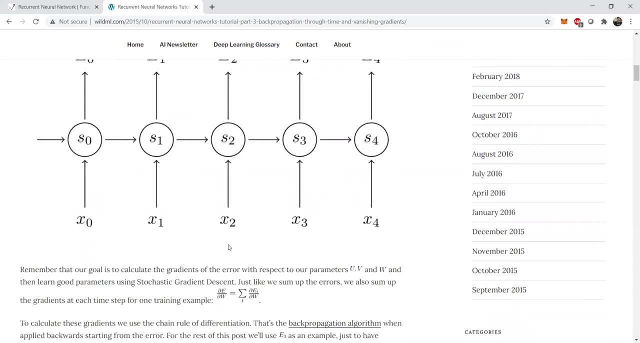 we want to reduce the amount of errors. we are effectively using this loss function that is given over here, our cross entropy loss, as our effective loss function and we want to minimize the error on this particular loss function. so in this case we want to find the minima for the. 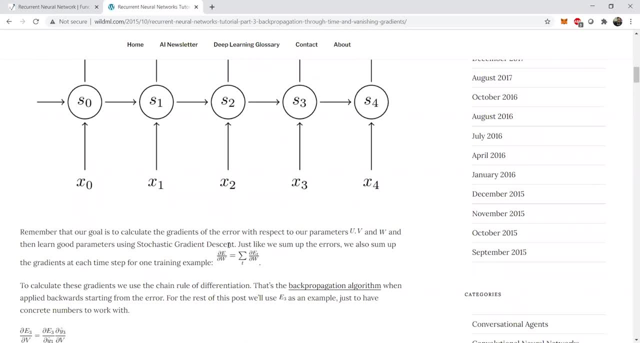 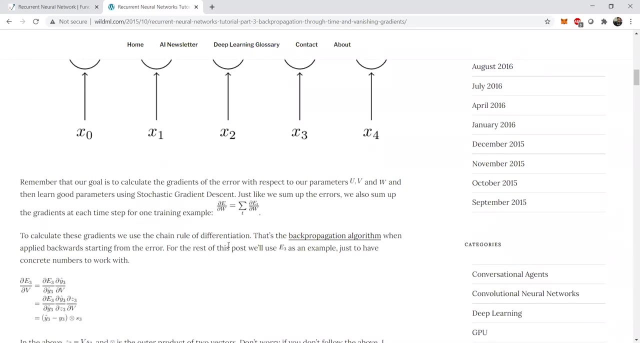 particular curve. in general, in calculus, if you want to find the minima, we generally do differentiation and in this case we want to do differentiation with respect to the weights because we want to update the weights for which are present in our loss functions. so in this case we will be going through the gradient descent algorithm because 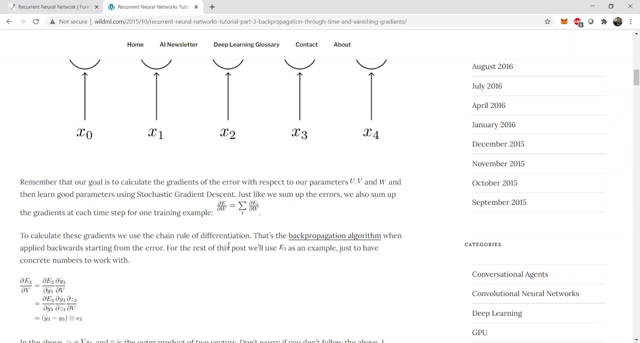 the gradient descent is the most basic algorithm and there is another variant called the stochastic gradient descent, where we sum up the errors for each of the time- you know each of the descent steps- and then we update the weights. either we increase the weights or decrease the weights. 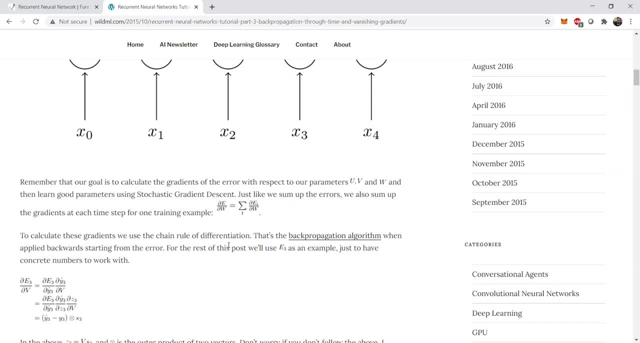 depending upon the, upon our errors. so generally the rule becomes d e by d w, where d is the error. uh, we have a summation of d e t for d w t. now. we have mentioned that propagation through time effectively takes place through time. so in this case we are doing all the summation of the weights. 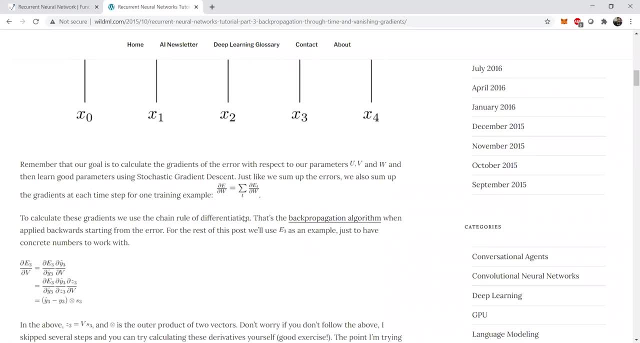 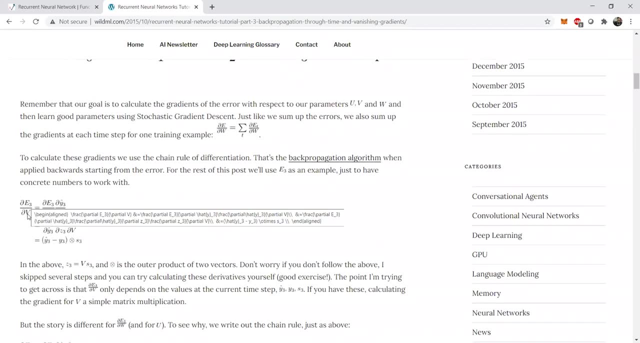 in stochastic gradient descent through time. so this is how the back propagation algorithm works through time right now. uh, if we, if we consider this equation very closely, we want to calculate the derivatives with respect to v, because v, if we, if we see this equation, we have a max of v times. 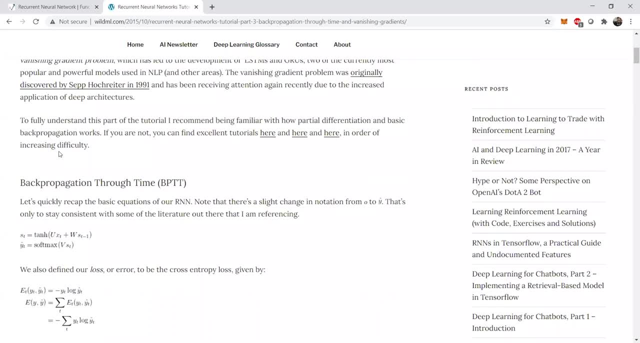 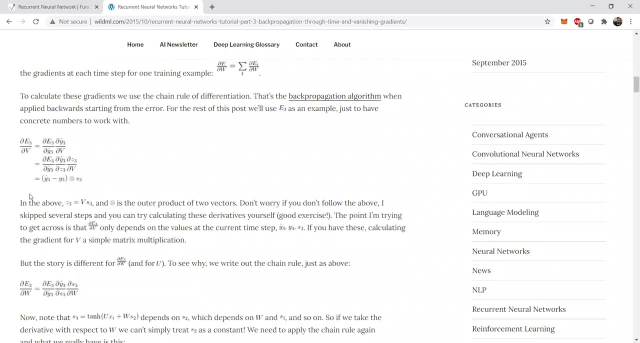 the st, where v is the sum of the weight of the gradient descent. so we have a sum of the weight of the gradient descent, is a weight. now if we were to apply this uh gradient descent differentiation on with respect to uh v, we have to do chain rule because directly e of e of three is not a function of having 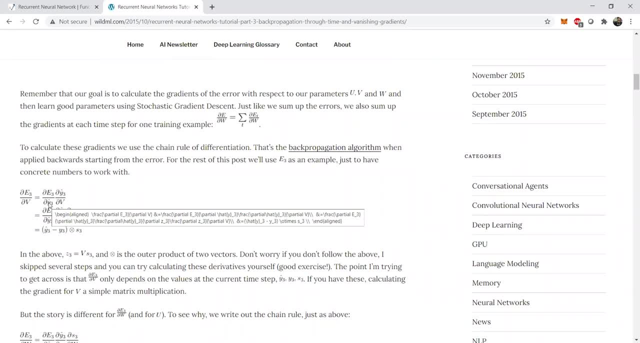 v as an input or an input feature. so we make the chain rule um in this case, because we want to first do derivative of e3 with respect to y cap, y cap 3, and then we do the derivative of y cap 3 with respect to v, because v is, just in case, present as an input feature in y cap 3, but e3. 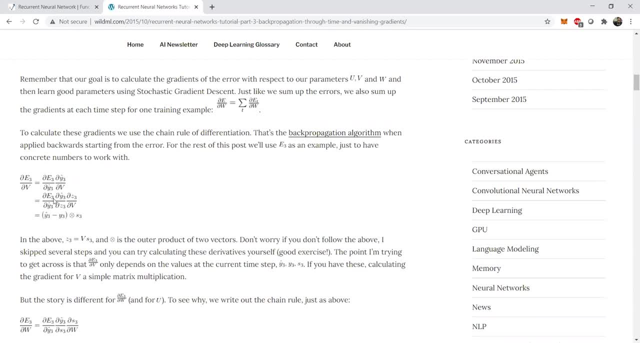 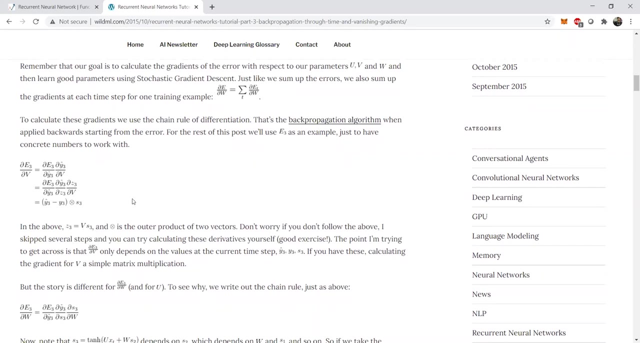 does not have that. so in this case- this is why the intuition of chain rule comes into the picture- we first do the derivative with respect to y cap 3, then we do the derivative of y cap 3 with respect to z3 and z3 with respect to v. now, what is z3? z3 is nothing but the v of s3. right, because v. so if 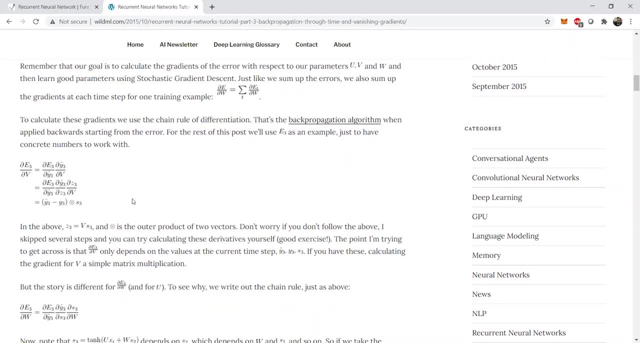 we are understanding with the chain rule concept. the chain rule is: if a function label is not present in a particular equation, then we cannot do derivative with respect to that particular, so with respect to that equation, and then we again decompose that equation into further steps until the smallest part contains that particular label. so that is what the intuition comes into. 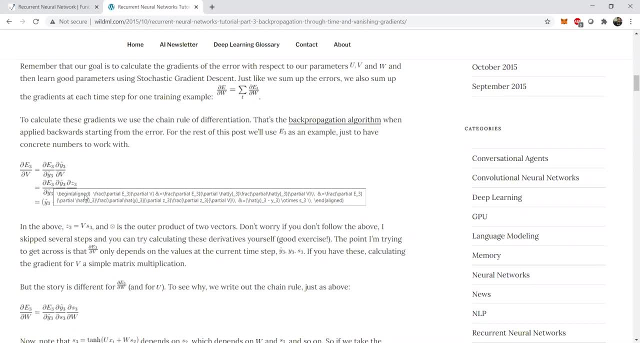 the picture. so d, e by d, y, cap 3, and then we do this chain rule, uh, we make the functions, uh, you know, having the same common part, that is the v, and then we, back, then we apply this chain rule again with respect to d, z3 and dv. so, effectively, if we, if we were to do this in our own notebooks, we will. 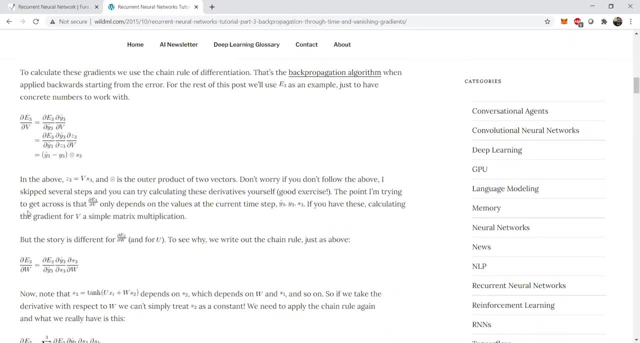 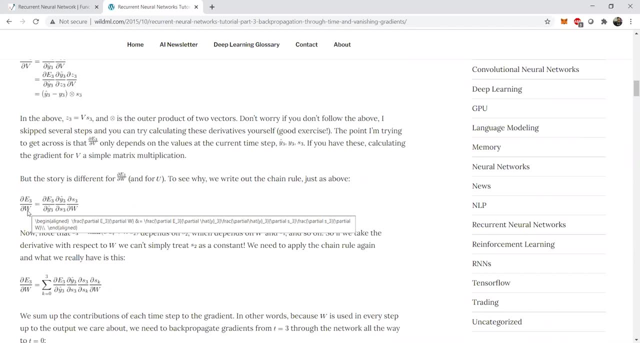 and understand it in a more clear manner. similarly in this case we do the derivatives for w. if we recollect, w was also with w h and w x h. so for these two bits also we have to do partial derivatives. that that means the chain rule, so d e 3 by d y cap 3 and then d? y cap 3 by d s 3 and then 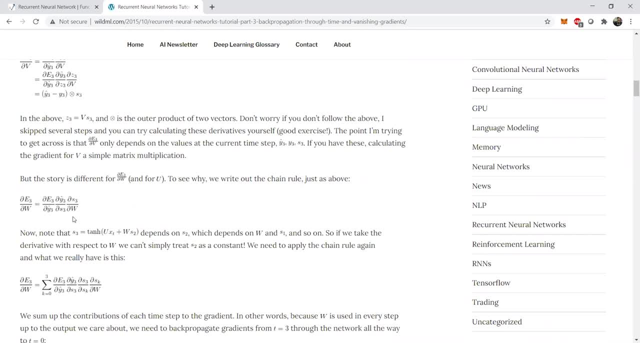 d s 3 followed by d w, because in the- in our case we d y cap 3 does not have any input feature with respect to w. so in this case we have to first do the derivative with respect to s3 and then we can move forward with ds3 and dw, where s3 is given by the tanh of the input features that we 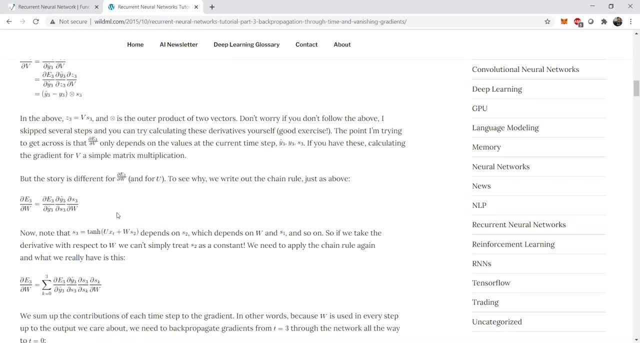 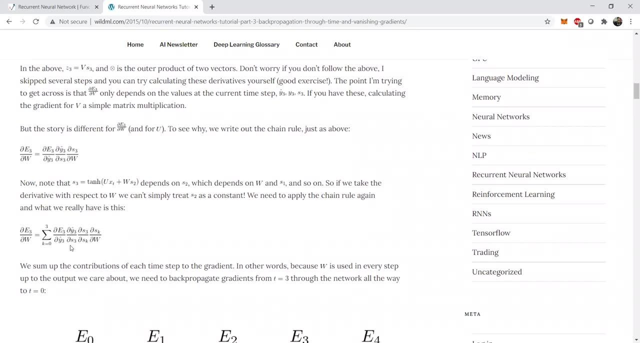 saw earlier in the forward pass and this step of back propagation and gradient descent actually actually continues, and this is where the summation of the weights with respect to the different timestamps it comes into the picture. so if we were to do with respect to dw, we can see that. 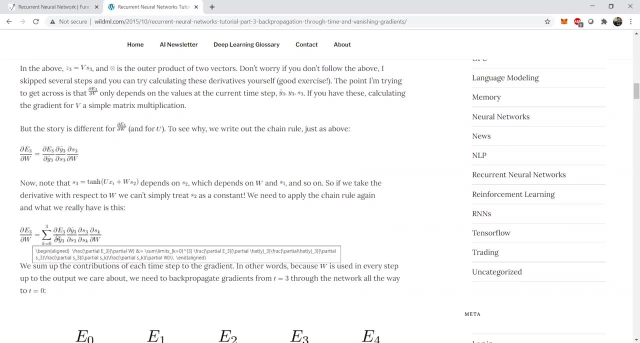 this chain rule actually elongates in a very long, long chain. so we have d e 3 given by uh cap 3, and this chain actually goes on until we get dsk by dw. so, um, this is where one of the important drawbacks of rnn comes into the picture, as well as one of the most important facts of 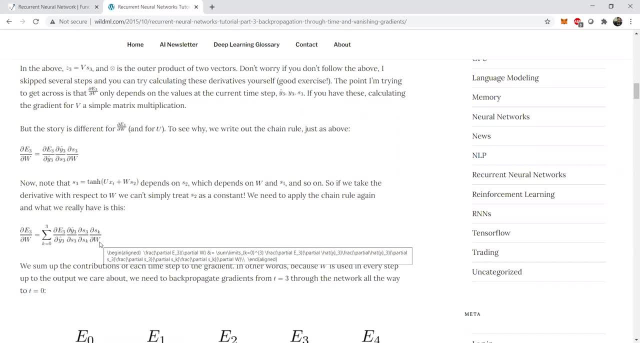 having an rnn. so you can see that if you, if you continue doing applying partial chain rule on these equations, the chain rule equation becomes very large and this is continued to back, propagated through time at for each time step. this is pictorially represented in this case. so you have 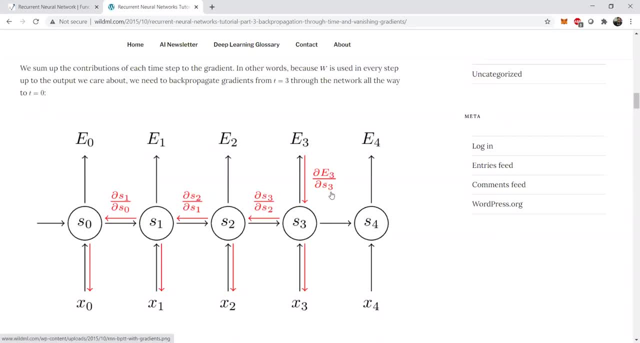 we see that first we are doing the derivatives with respect to de3, with respect to ds3, and then we are taking the outputs for that and we are back propagating it to s2. so we are effectively taking the derivative of s3 with respect to s2 and then we are again taking the derivative with 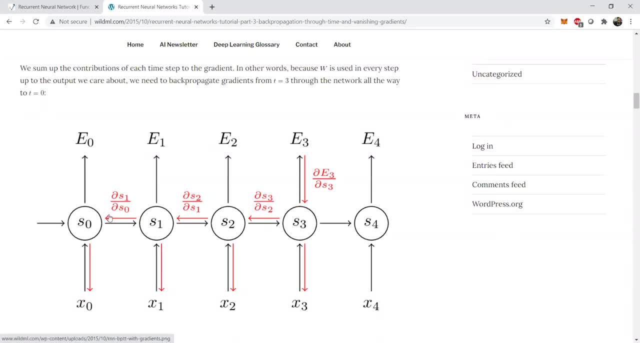 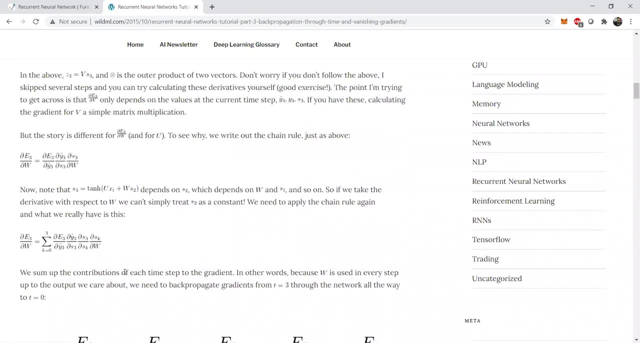 respect to s2, with respect to s1, and then this process continues until we reach the source. that is the first step, that is the s0 step. so this process effectively continues for all the times. in recurring neural networks we just saw- to summarize, we saw two things. 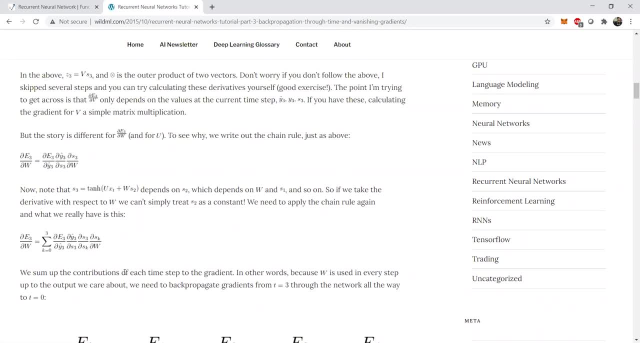 first is the recurrence pattern, where we have an equation, a tanh activation, activated equation of weight vectors multiplied with h. that is the time step plus the input features xt, multiplied with some weight vectors, w, xt, and then we apply tannys on it and after that we have to get the 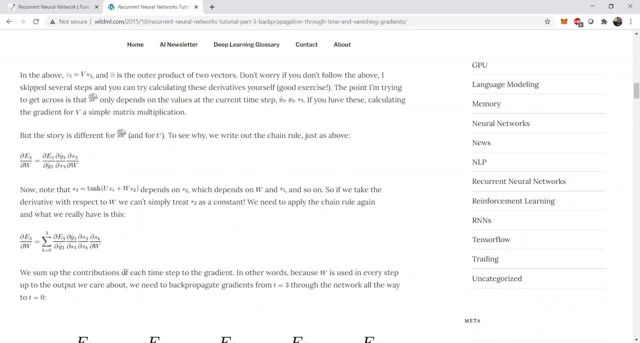 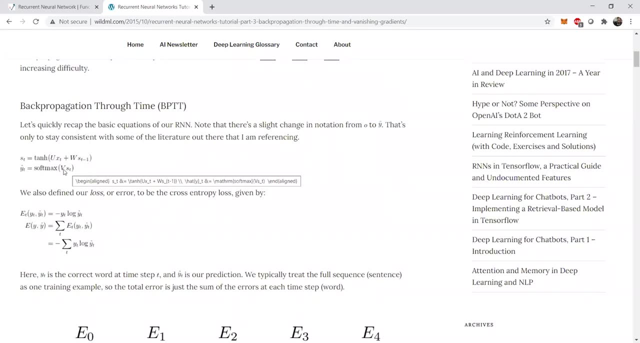 output for that recurrent neural network. in the forward pass we compute the yt which is given by the softmax activation of the vt dot st. so in this case case, if we just go back to the previous equation, we will have why cross yt ht. so in this case we 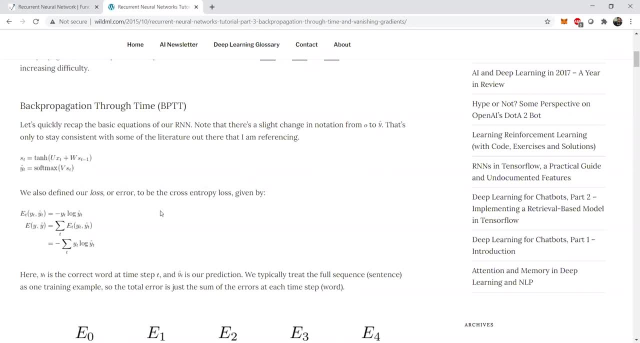 get the yt by having in the forward parts. now, in this case we also want to do minimize the error. so in this case we first devise the loss function, in our case that is the cross entropy loss that is given by summation of yt into log times, y, cap t, and then we want to do partial derivatives. 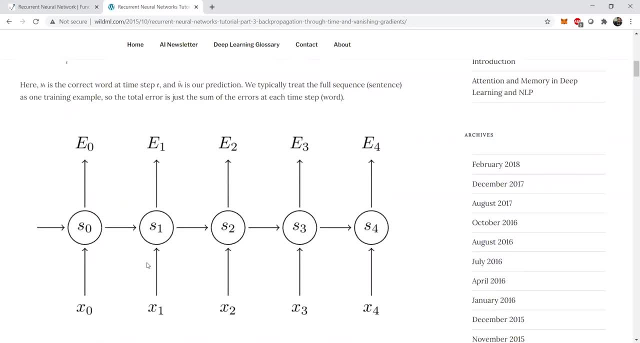 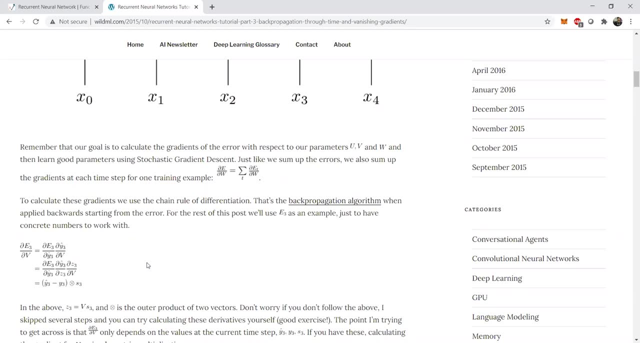 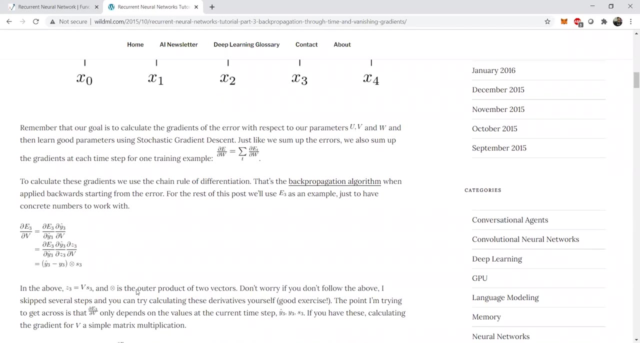 because we want to perform minimization or gradient descent, to minimize our errors, right. and that is where the back propagation through chain rule, through time, comes into the picture. and this is the effective equation for back propagation where we have d? e with respect to the weights, with summation over time, and in this case, if we expand this equation, that is the 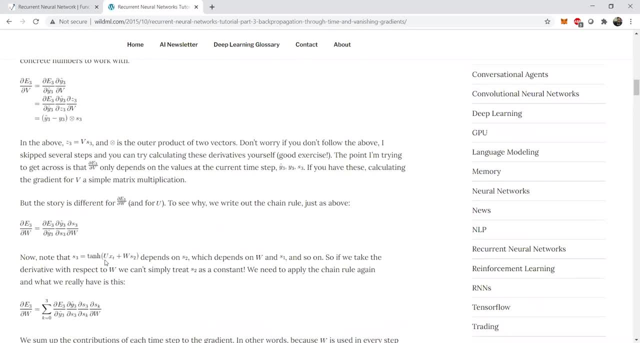 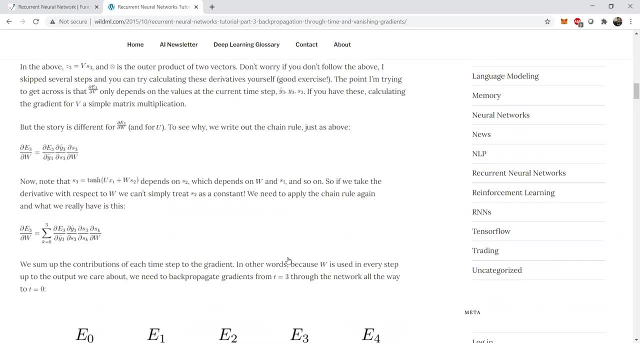 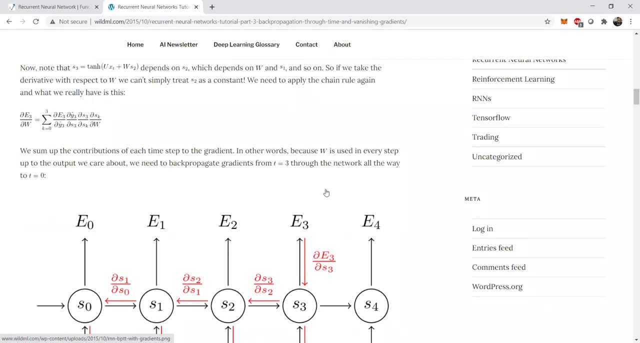 chain rule differentiation equation. we will see that this equation of expansion is getting really large and that is where the intuition for having these kinds of uh gradient descent for each time step comes into the picture. so for in this we can see in this image: first d e3 with respect to s3 is computed. the output of that is computed. 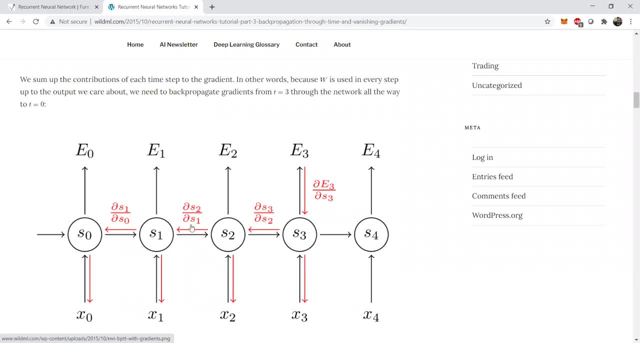 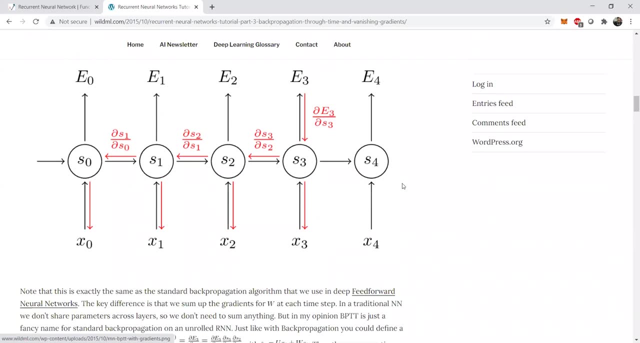 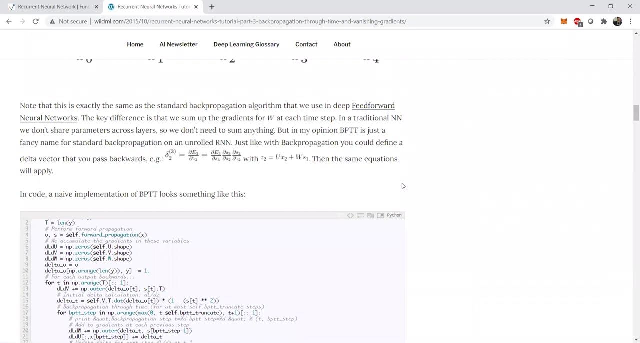 is again done, derivatives with respect to s2, that is again done, derivatives with respect to s1, and this process actually continues, right, and if we move forward, we have a vanishing gradient problem in rns, which is a very, uh, hard problem, because if we, if we recollect, using this equation, where 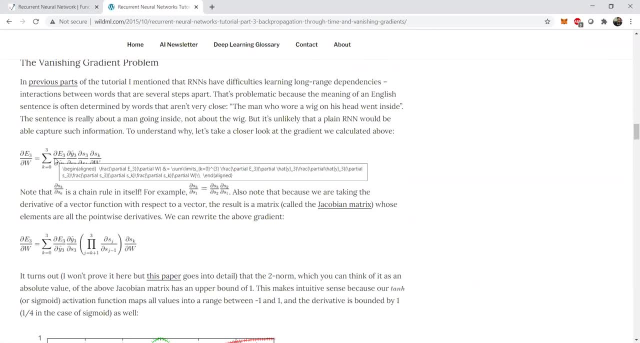 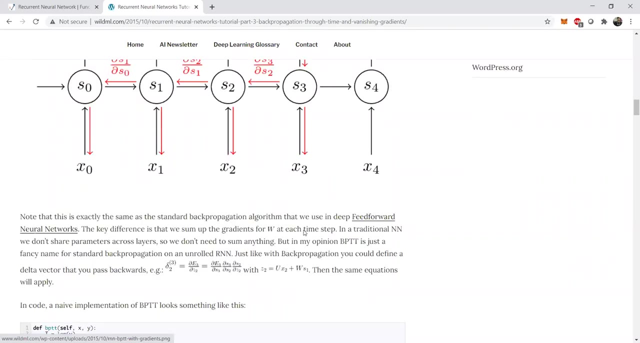 i mentioned that the chain rule differentiation equation actually becomes large and this is effectively done, shown in the picture over here. so if you have thousands of units of recurrent neural networks, different neurons, one after the other, you can see that the gradient is computed at each and every step. and when you are computing gradients, the gradient actually 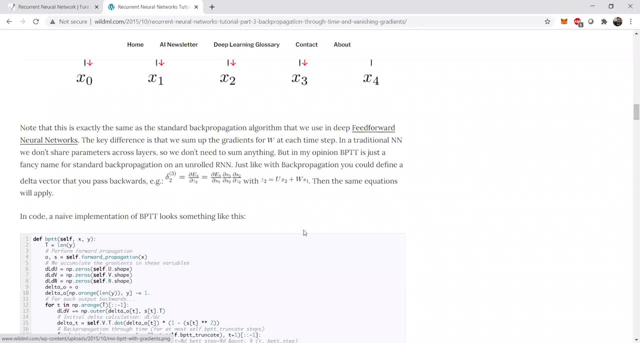 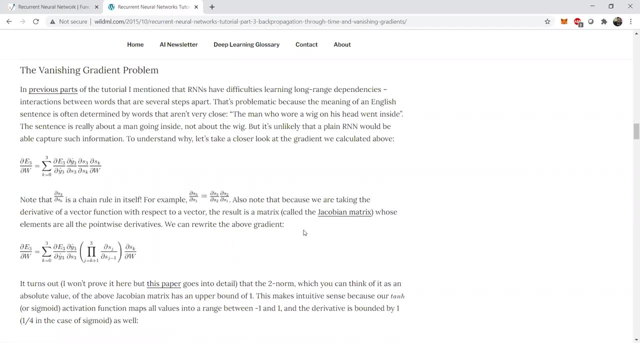 becomes very, very, very, very small at each and every differentiation step. so it becomes literally very uh hard to know whether the gradient, whether the gradient drop, is there or not. in most of the cases the drop becomes so, so small, so so minute that it becomes impossible for the weight update to take place. so in that case the weight update becomes really really small. 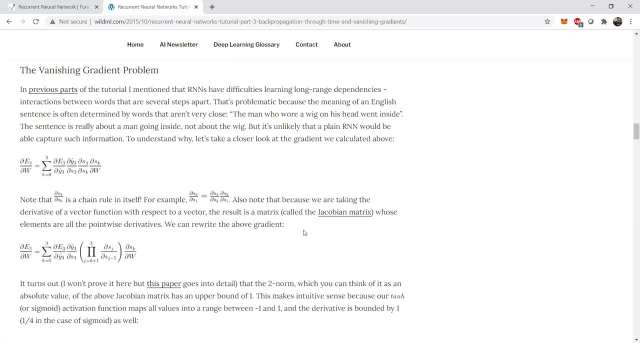 and the learning is not improved. learning does not improve as the epochs go on. so in that case we are left with something called as a vanishing gradient problem, where the rnn does not capture any information, any more information, and there is something called as a damping of the uh of the 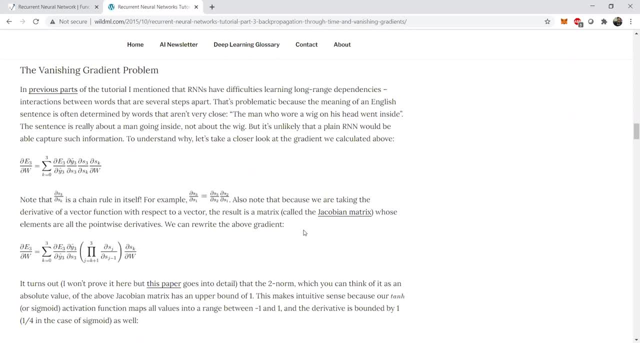 weights. that is taking place because the weight updates are not taking place because the gradients are are very, very small, are negligible in that way in in numbers. that is where you know some important features, uh, like lstms and gru's, are coming to the picture, which we will cover in the next few topics, but in this case, uh, this is the. 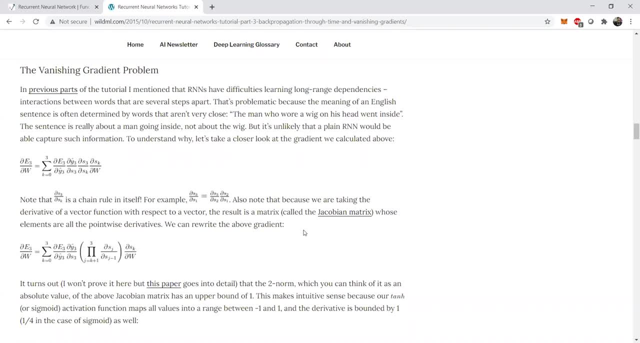 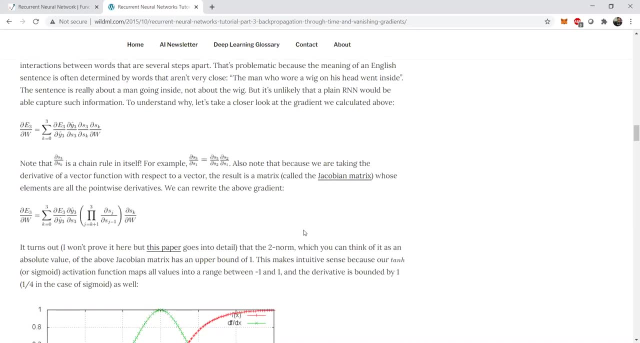 drawback of the rns because of the chain rule becomes really large, it becomes difficult for to understand uh where the update is taking place and uh effectively in. in the concept of tensor, this is computed as a jacobian matrix, right, and in this case this jacobian matrix is effectively a. 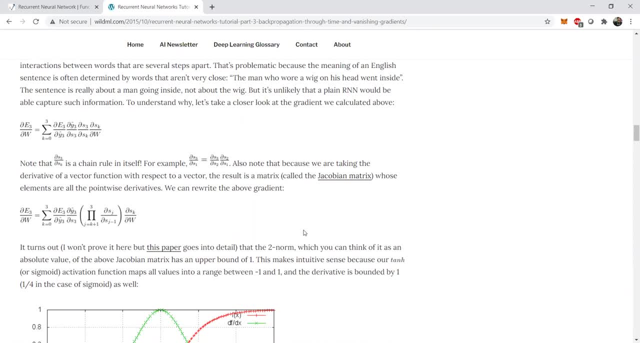 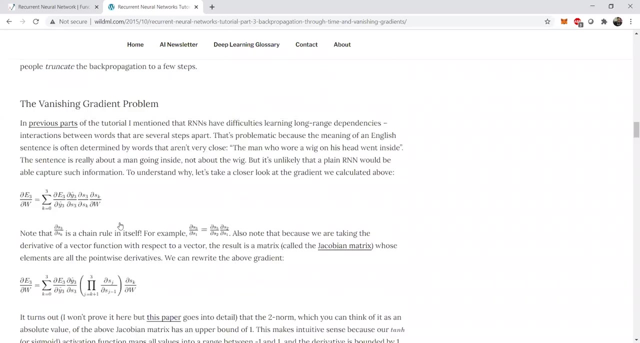 uh done by the differentiation of all the individual weights present in the particular uh tensor or a particular matrix right, and this particular equation is a unrolled version of this particular equation where we have a product of dsj given by the dsj minus one, which is effectively 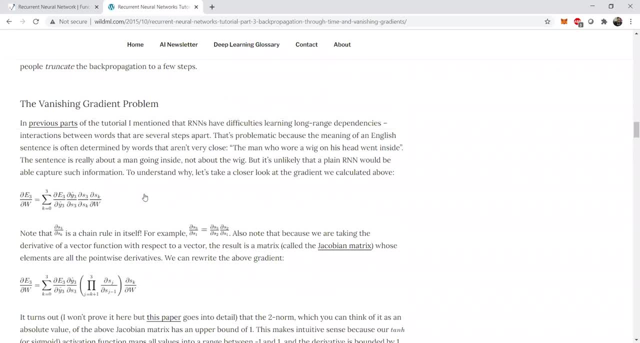 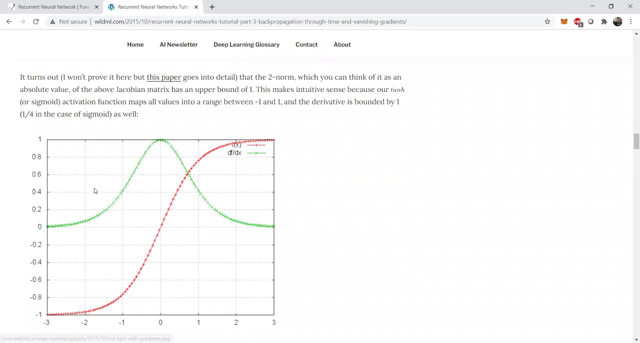 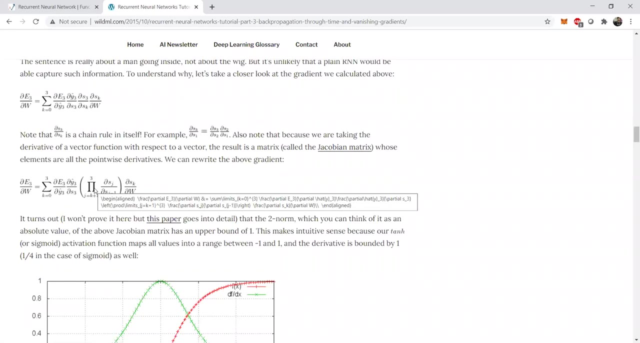 the loop from here. as we increase the number of layers inside neural layers, we can see that this step continues for a longer period of time, and this is where this particular part um actually helps to decompose the weights and the gradient is not properly attained. the gradient change is 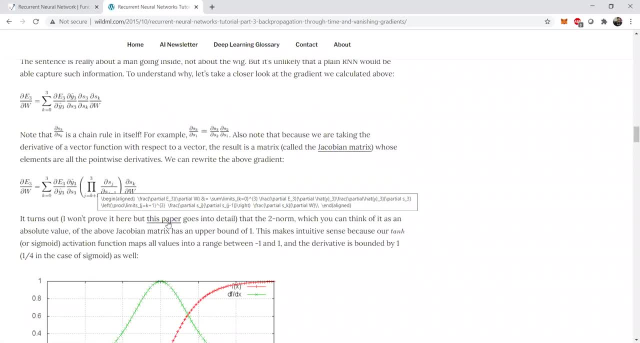 not properly attained and there are several resources this paper also has provided in this link- also has a very mathematical detail as to why this gradient vanishing gradient problem comes into the picture. and that is all mostly what i wanted to cover about recurrent neural networks in general. so, to summarize, recurrent neural networks are highly- uh, sophisticated neural. 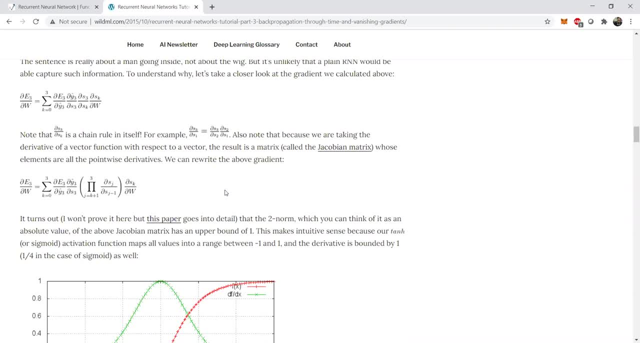 architectures which can be used for sequence classification, sentiment classification, any nlp tasks in general, and they form the base for all the advancements that have been their current uh in the present time instant. so they use the recurrence relations, they use the information from the previous time steps and there are two passes. one is the forward pass where we compute the teenage activated uh.